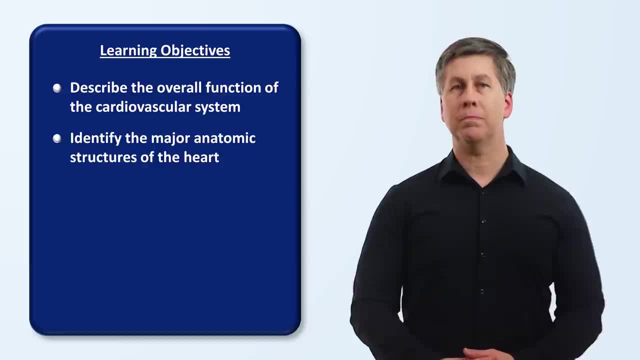 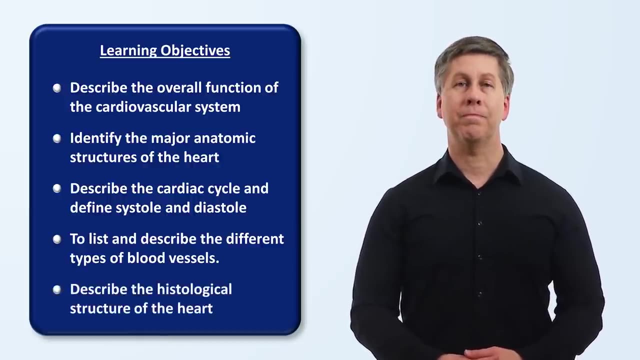 and the primary components of the conduction system. You'll be able to describe the cardiac cycle, including the definitions of systole and diastole, to list and describe the different types of blood vessels and to describe the histologic structure of the heart. 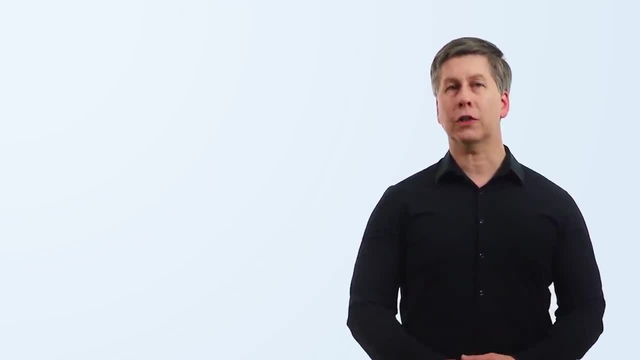 In short, the function or purpose of the cardiovascular system is to pump blood around the body. But why? The simple answer is the delivery of oxygen. Deoxygenated blood, that is, blood that's relatively lacking in oxygen, is pumped from the heart. 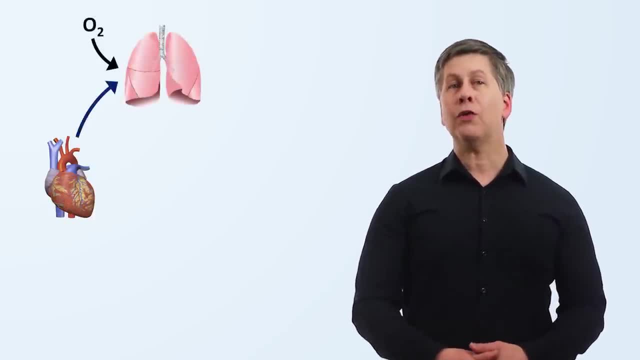 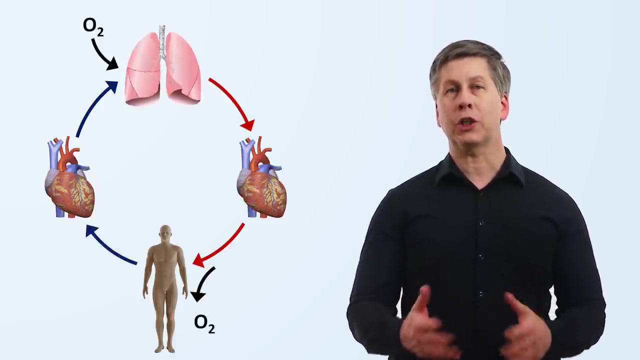 to the lungs, where oxygen is picked up. The now oxygenated blood returns to the heart, from where it's pumped to the rest of the body, at which point the oxygen is offloaded within other organs and tissues. The oxygen is an essential part of cellular respiration. 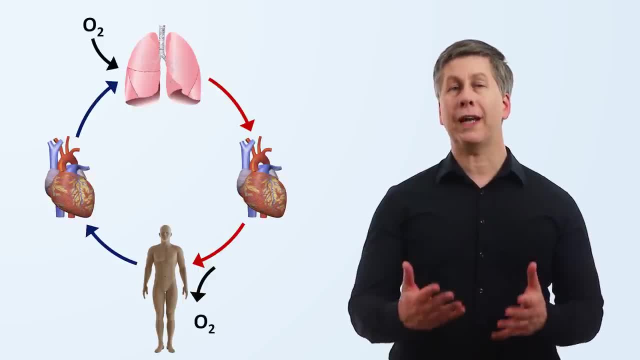 This is the process by which cells generate energy, storing ATP from glucose and other molecules containing chemical potential energy. But the movement of oxygen is just part of the story. Blood carries a lot more than that, For example, waste products, Most notably carbon dioxide, which is a byproduct of cellular respiration. 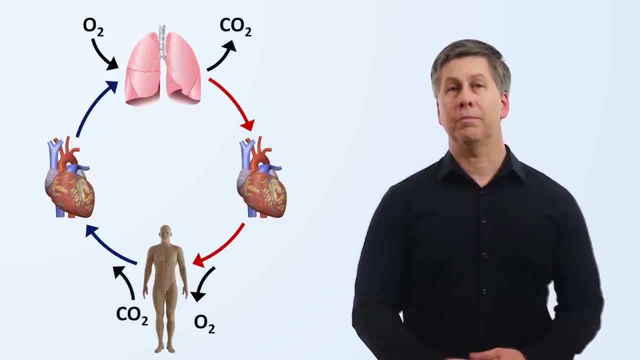 and which the heart must pump back to the lungs to be exhaled. Blood carries other metabolic waste products to the liver, such as bilirubin and lactate, for processing and, in some cases, elimination from the body, for example in bile. 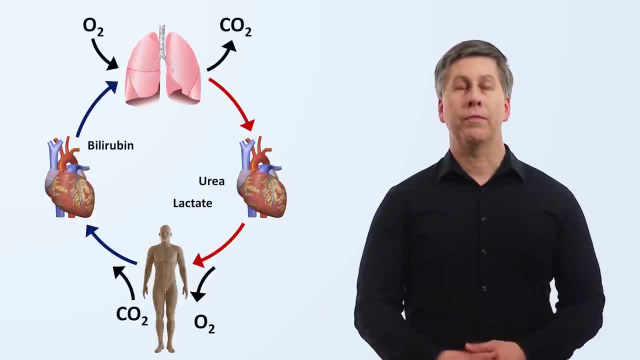 It carries urea to the kidneys to be excreted in the urine. Blood transports electrolytes, glucose, fatty acids and it transports hormones like insulin and cortisol that allow one part of the body to send signals to another. And it carries essential components of our immune system. 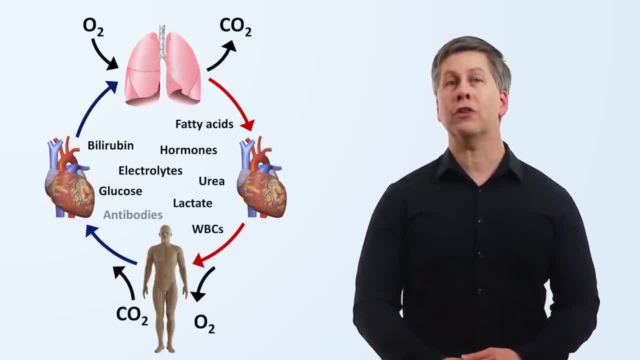 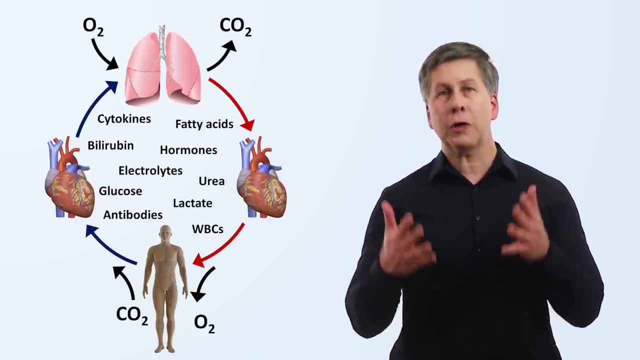 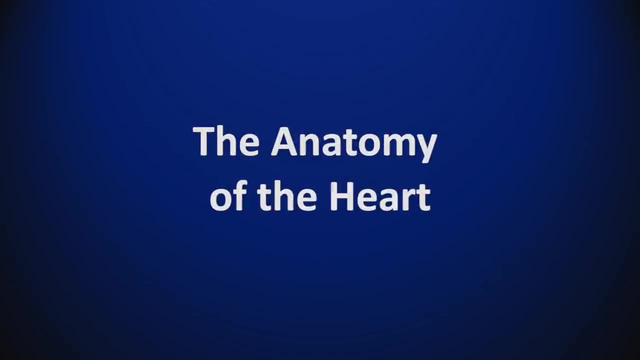 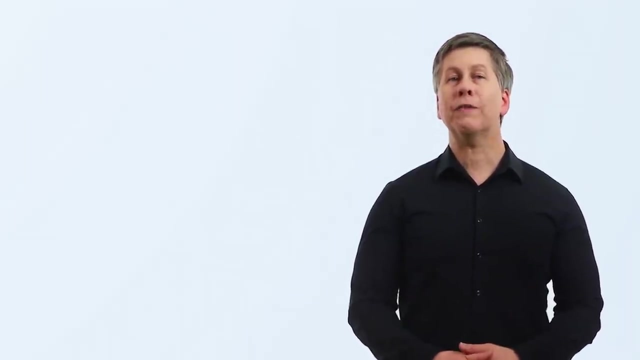 like white blood cells and proteins such as antibodies and cytokines. So while it's true that the circulation of oxygen is the single most important function of the heart, it is far from the only necessary one. To understand how the pumping mechanism works, let's first focus on the gross anatomy of the heart itself. 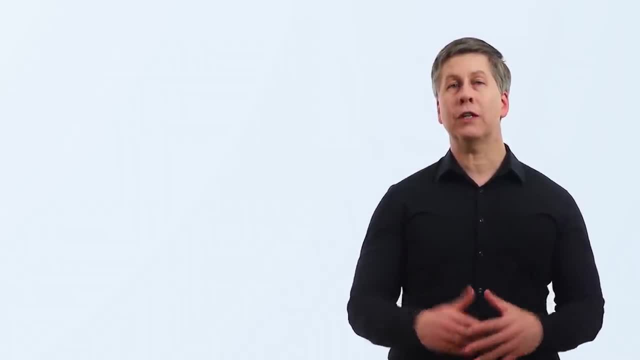 The heart is a surprisingly difficult structure to represent. with a two-dimensional picture, No matter what angle or cross-section is viewed, at least one notable structure will be hidden behind others And kind of like a map of the world. there is no two-dimensional view that accurately represents 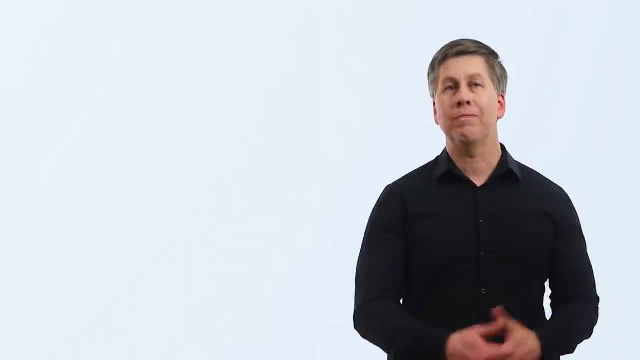 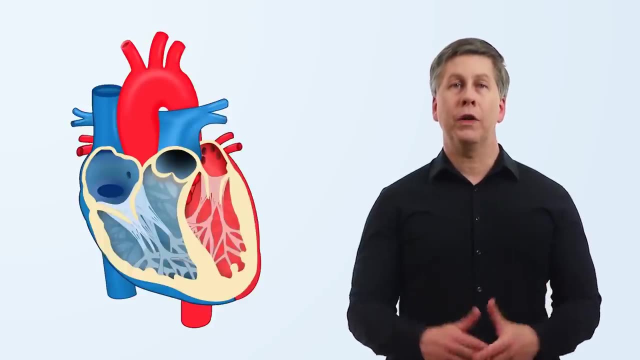 both the relative size and location of the chambers. I'll start with this view, but I'll switch around to other images as needed. On the most basic level, the heart's physical structure consists of four chambers surrounded by muscular walls, four valves. 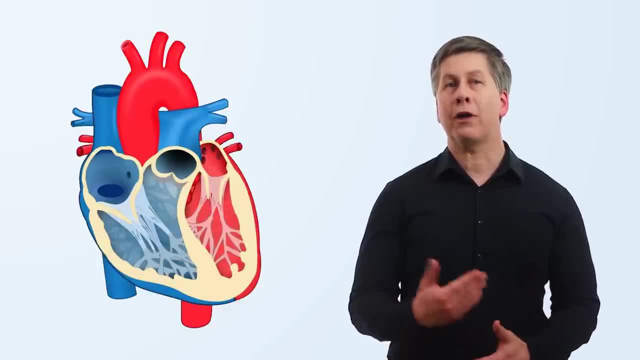 a handful of so-called great vessels and a number of minor vessels. To give a lay of the land, I'll walk through the path that blood takes as it returns from the body in its deoxygenated state. First blood arrives in the chamber called the right atrium. 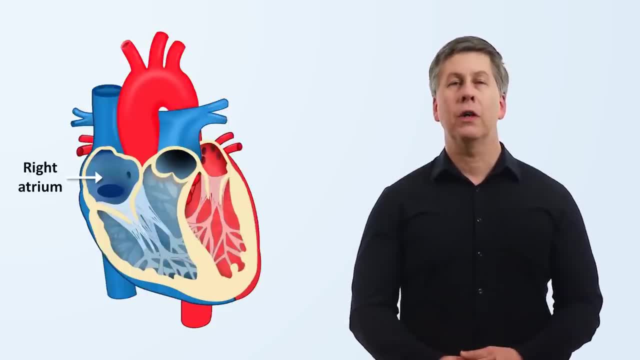 blood can reach the right atrium through one of three paths: All blood returning from above the diaphragm enters via the superior vena cava. all blood returning from below the diaphragm enters via the inferior vena cava. and most blood returning from the heart muscle itself. 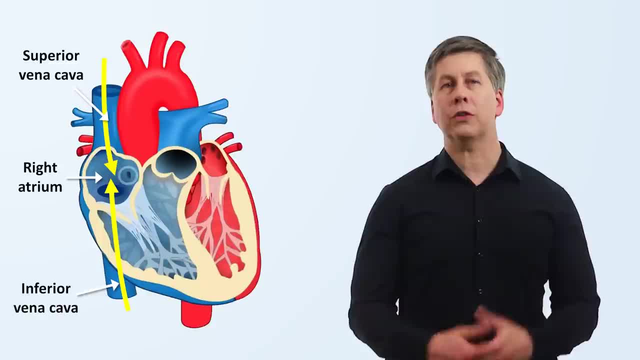 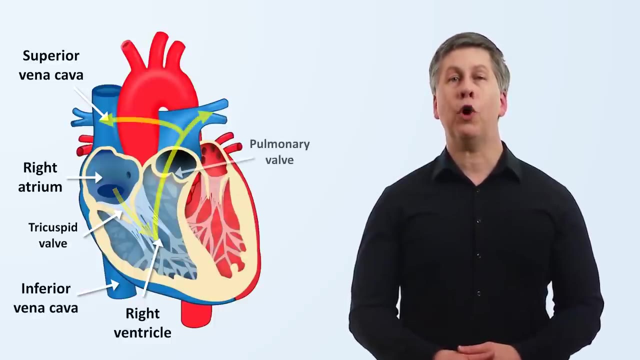 enters the right atrium via this much smaller vessel called the coronary sinus. From the right atrium, blood travels through a valved opening called the tricuspid valve into the right ventricle. From the right ventricle it travels through another valve called the pulmonary valve. 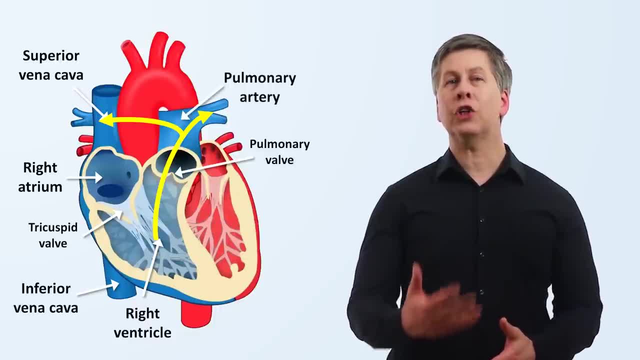 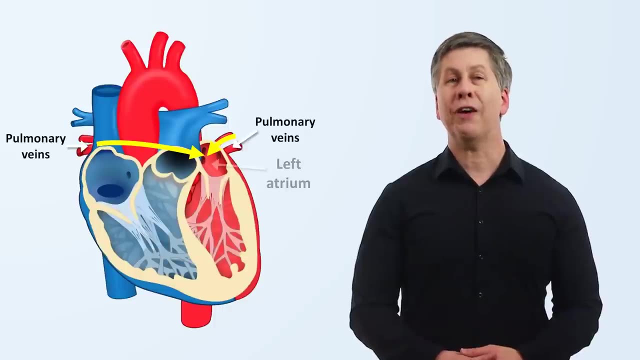 into the pulmonary artery, which carries the still deoxygenated blood to the right and left lungs, where carbon dioxide will be offloaded and oxygen will be picked up. The oxygenated blood returns to the heart via one of four pulmonary veins, bringing it to the left atrium. 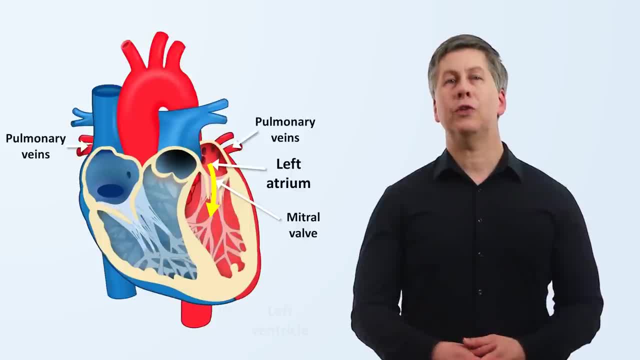 From the left atrium it travels through the mitral valve into the left ventricle. From the left ventricle, blood then exits the heart through the aortic valve, which is hidden behind the pulmonary valve in this particular view. 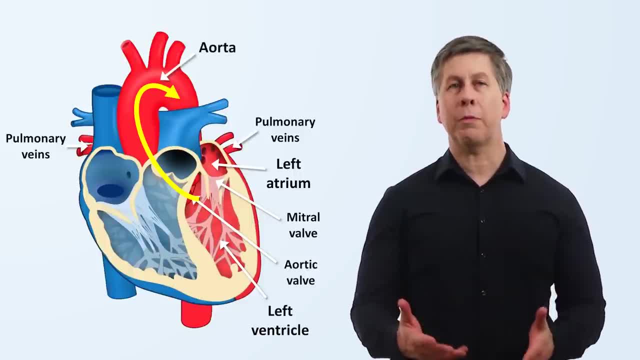 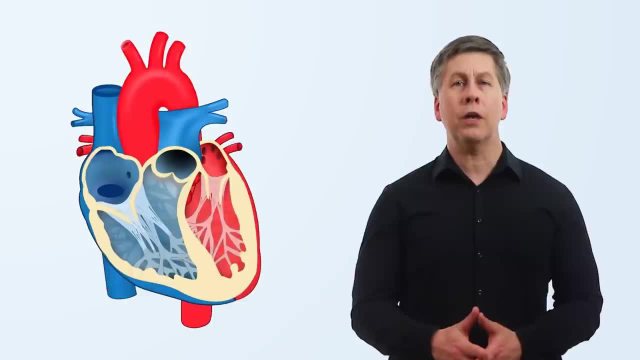 And then it travels via the aorta to the rest of the body. This sequence of steps from the vena cava to the aorta is separated into two segments by the lung, with the right side of the heart containing deoxygenated blood. 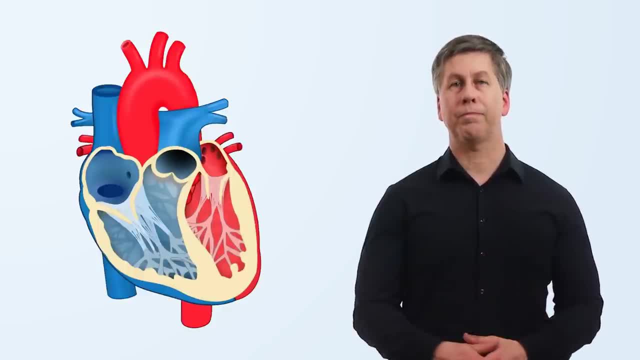 and the left side of the heart containing oxygenated blood. The right and left atria are separated by a relatively thin interatrial septum hidden here behind the right ventricular outflow tract, while the left and right ventricles are separated by the relatively thick and muscular interventricular septum. 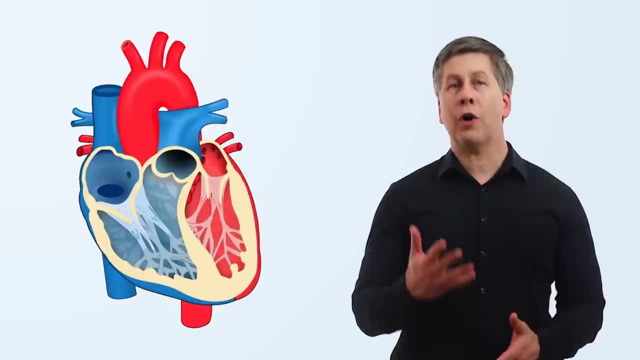 As a side note, while almost all diagrams of the heart show the right heart in blue and the left heart in red, deoxygenated blood is not literally blue, but rather more of a maroon color. Also going back to my previous comment about how, 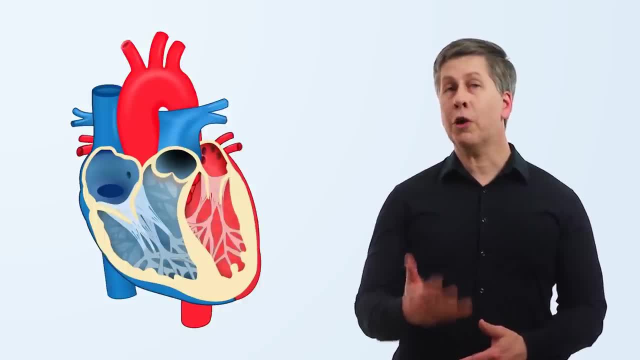 no single view of the heart is perfect. this view makes it appear that the right heart is larger than the left, when in reality the left is larger than the right. It's just that the left heart sits somewhat posterior to the right when viewed from this angle. 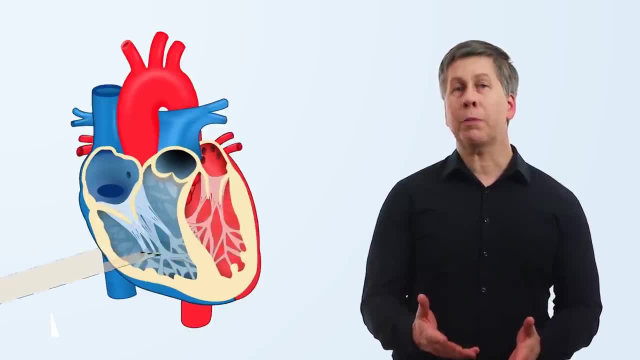 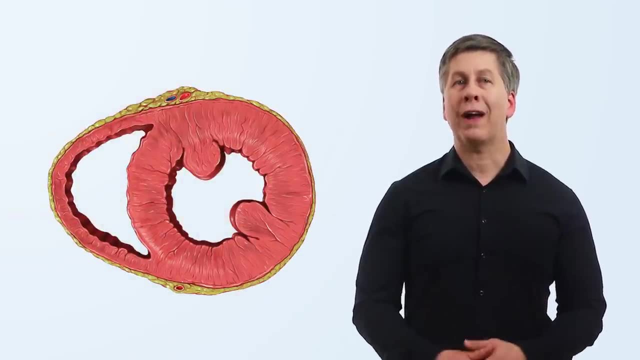 If we look at a cross section of the heart taken along this plane, we get a better idea of the relative volume and shape of the ventricular chambers. The large round, thick-walled one is the left ventricle and the smaller crescent-shaped one is the right ventricle. 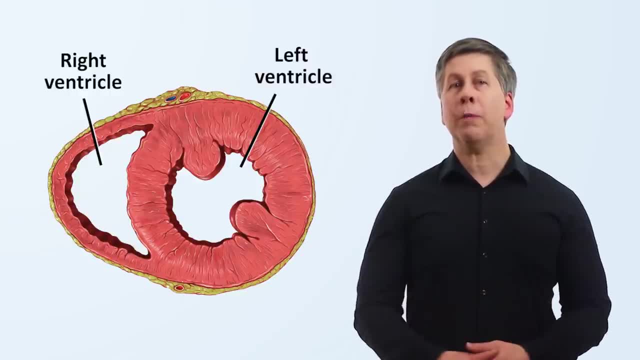 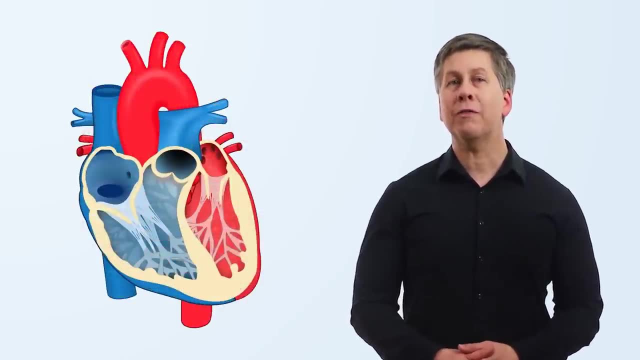 The left ventricular wall needs to be much thicker because it pumps against much higher pressures than the right one does. Back to this view. let's discuss the valves a little more. The valves consist of leaflets or cusps that allow movement of blood in only one direction. 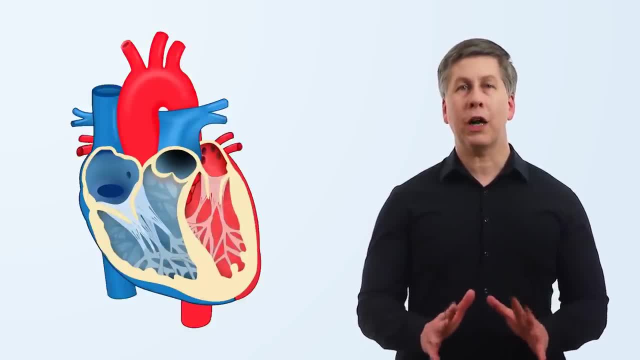 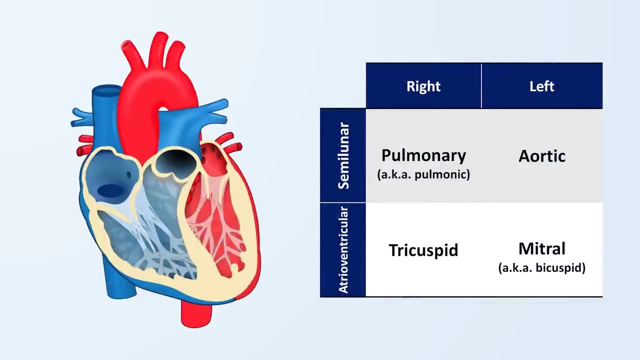 All of the valves normally have three cusps, except the mitral valve, which normally has two. Each valve belongs to one of the two sides of the heart- right versus left- and each has one of two structures: atrioventricular versus semilunar. 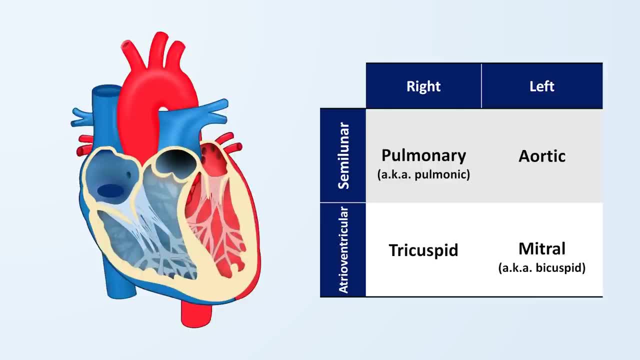 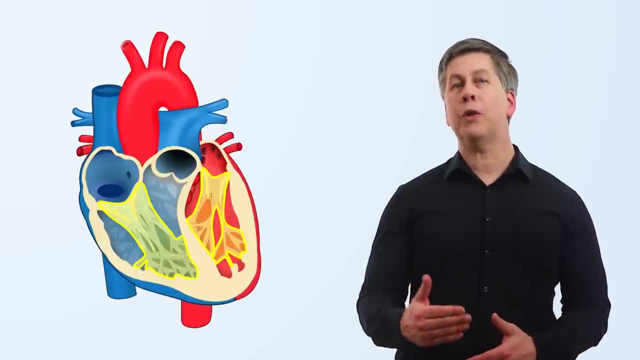 The cusps of the two atrioventricular valves are attached to fibrous threads called chordae tendineae or tendinous cords. These are in turn attached at the other end to the papillary muscles, which are conical projections from the walls of their respective ventricles. 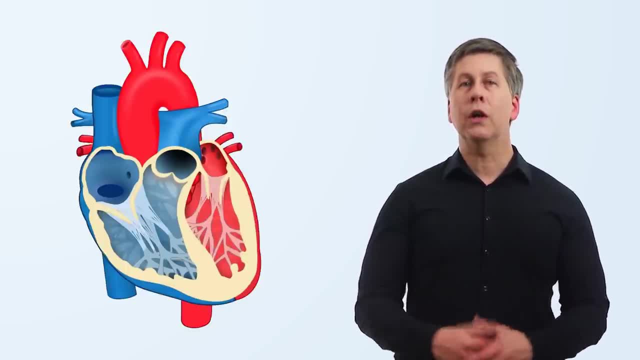 The purpose of the chordae tendineae and the papillary muscles are to prevent backwards movement of the valve cusps during the high pressures generated when the ventricles contract, which otherwise could result in the retrograde movement of blood from the ventricles backwards into the atria. 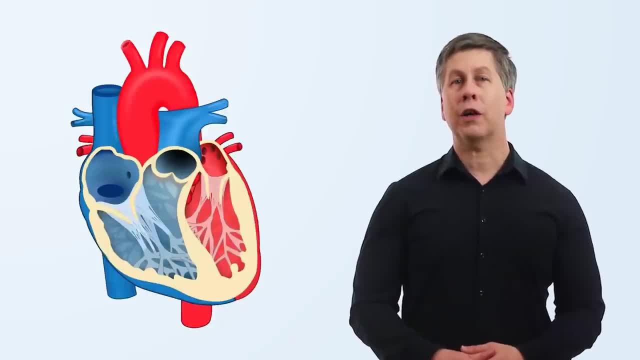 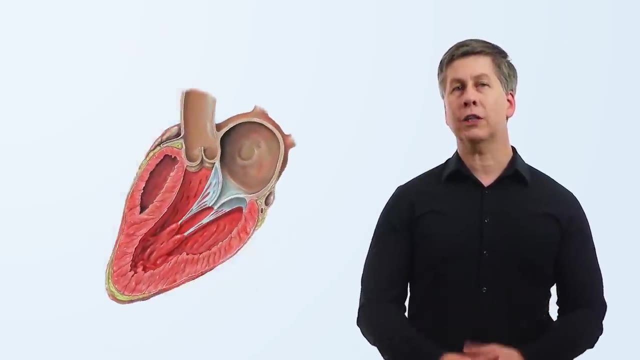 The semilunar valves, named because their cusps are reminiscent of half moons, are concave when viewed from above, They both normally have three cusps and no chordae In this classic cross-sectional view of the heart known as the parasternal long axis view. 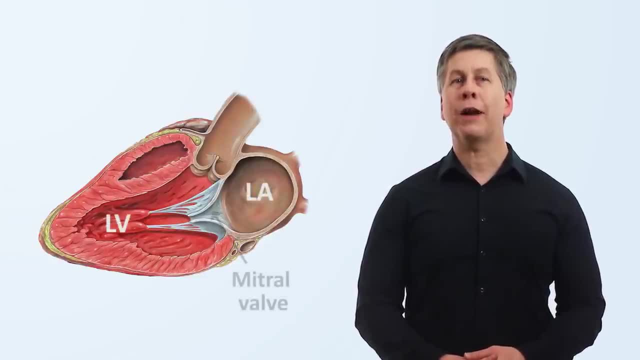 we can see the significant difference in structure between the mitral valve, with some of its chordae and one of the papillary muscles, and the adjacent smaller semilunar aortic valve. One final point to make about the valves is that, although it can be hard to appreciate, 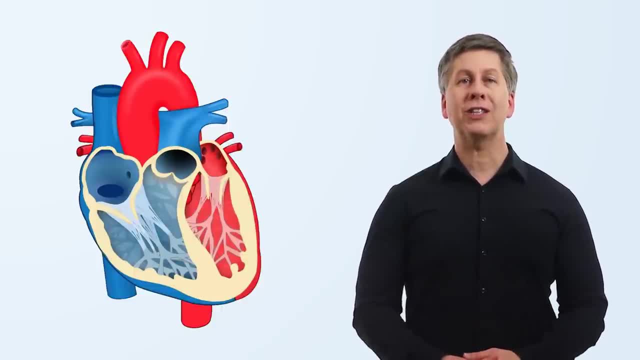 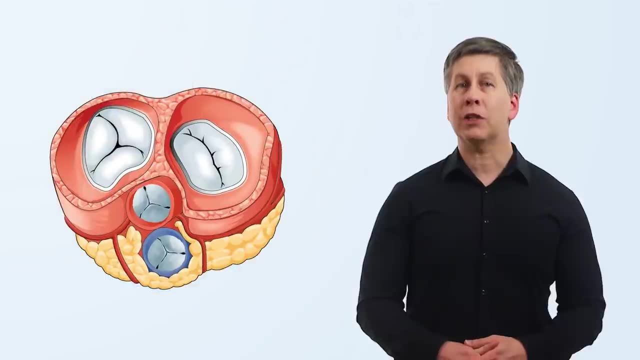 in most two-dimensional views, the four valves sit in close proximity in roughly similar plane to one another. This plane is composed of fibrous tissue that includes fibrous rings around the valve openings. These rings are stiff and they help to maintain the valve shape. 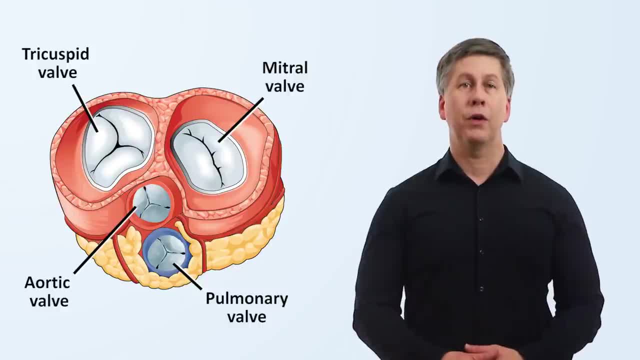 and provide structure to which the valve cusps can attach. More generally, this fibrous tissue functionally acts as the skeleton of the heart. It also is non-conductive of electricity, which is critical for proper regulation of the heart rhythm, as it funnels electrical signals. 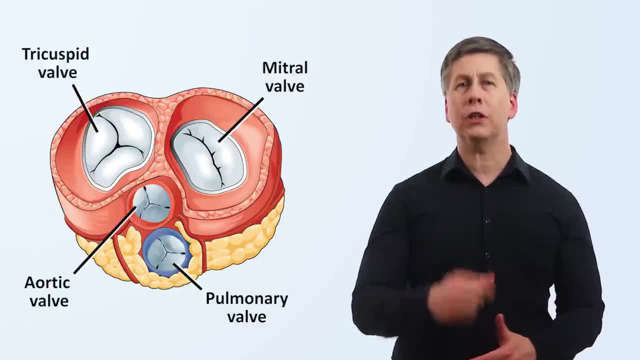 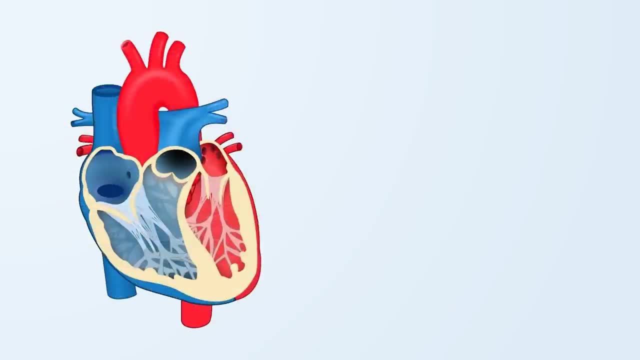 between the atria and ventricles to a relatively small location called the AV node, where it can be more easily regulated. Although I've already mentioned them individually to review, let me list the eight great vessels. These are the superior and inferior vena cava. 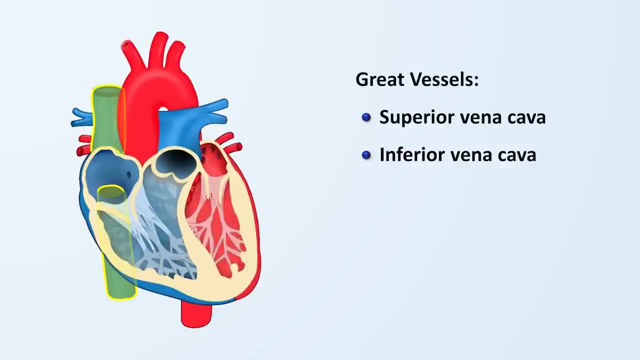 which bring blood from the body to the right atrium. the main pulmonary artery, which bifurcates into the right and left pulmonary arteries, which travel to the right and left lungs respectively. the aorta, which is the main artery of the body. 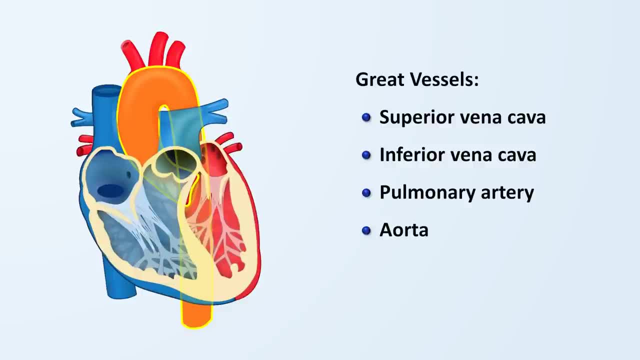 from which all other arteries branch except the pulmonary artery. It's often divided into four parts: the ascending aorta, which then loops up and posteriorly into the aortic arch, which continues downward and becomes the descending thoracic aorta, coursing posterior to the heart. 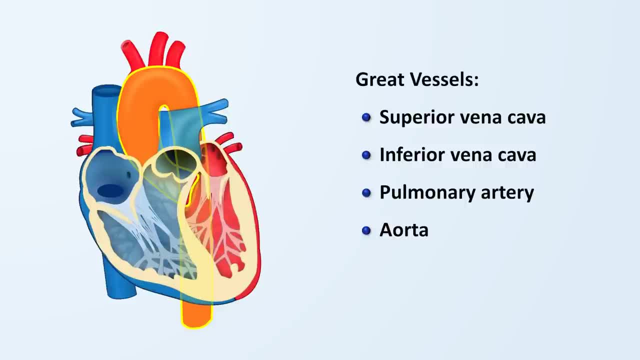 and once the aorta crosses below the diaphragm, it's known as the abdominal aorta. And last, the four pulmonary veins which bring blood from the lungs to the left atrium. And this brings us to the conduction system. 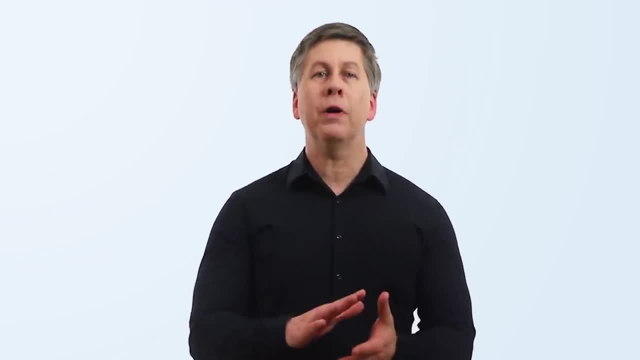 While we often think of the heart as primarily a mechanical pump, there needs to be some mechanism that tells each chamber when to contract and when to relax, And that mechanism is the conduction system, which delivers electrical signals to different chambers at different times. 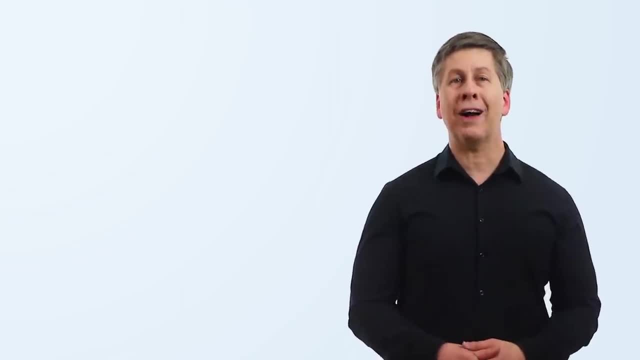 Electrical impulses normally originate within a specialized tissue called the sinoatrial node, SA node or sometimes just sinus node. It's located in the superior posterior aspect of the right atrium. The frequency of these impulses is governed by a balance between the sympathetic and parasympathetic divisions. 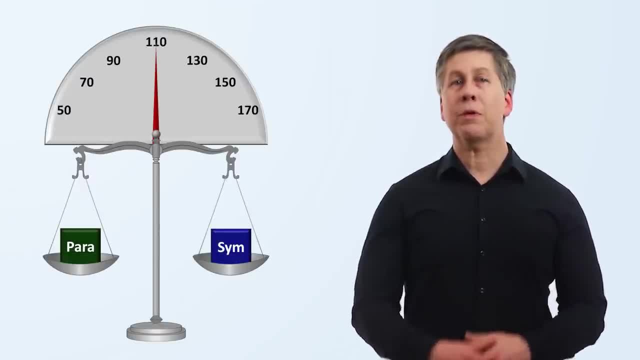 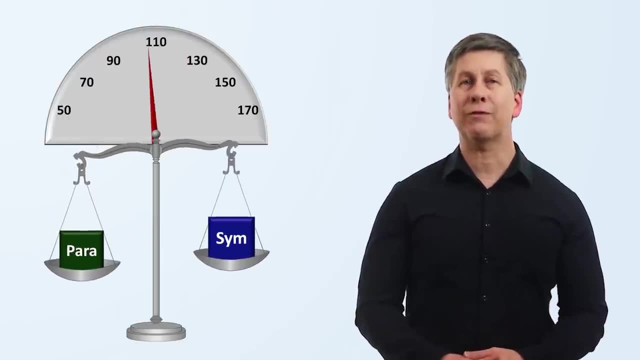 of the autonomic nervous system. The sympathetic nervous system tells the SA node to fire more frequently, while the parasympathetic nervous system tells it to fire less frequently. In normal, healthy adults, the balance between these two results in a resting heart rate. 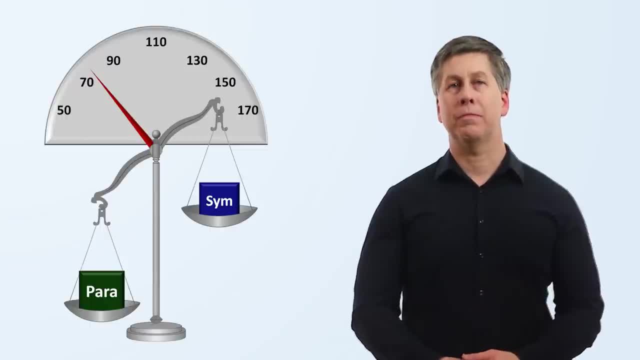 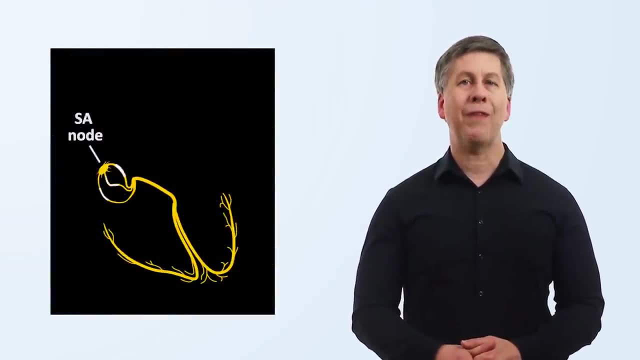 between 50 and 90 beats per minute. Electrical impulses fired from the SA node travel throughout the two atria, triggering their contraction and the ejection of blood through the AV valves into their respective ventricles. The electrical signal will next reach the atrioventricular or AV node. 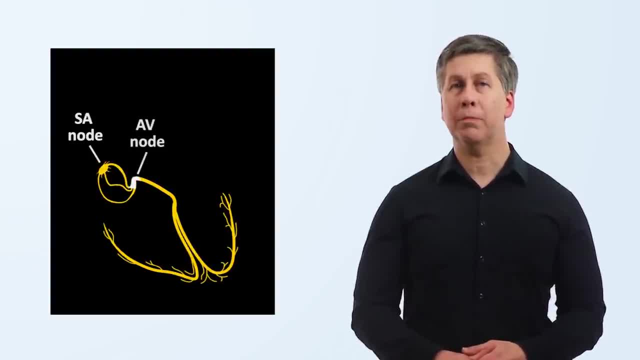 within the inferior part of the atrium. While the SA node can be thought of as the pacemaker of the heart, the AV node is more of a gatekeeper. As mentioned, it's the sole location in which electricity can normally pass from the atria to the ventricles. 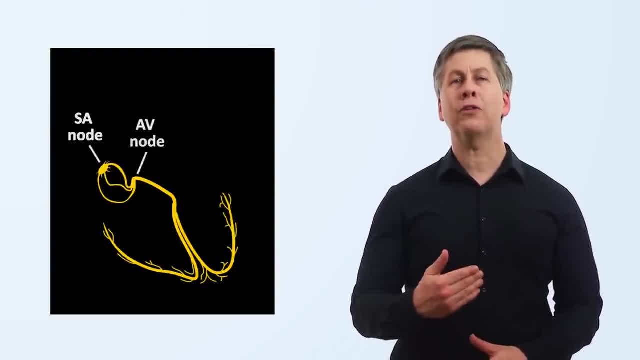 and it conducts relatively slowly, providing time for blood to move from the contracted atria into the relaxed ventricles. After holding up the signal by 100 or so milliseconds, or a tenth of a second, the AV node lets it continue through a band of conducting fibers. 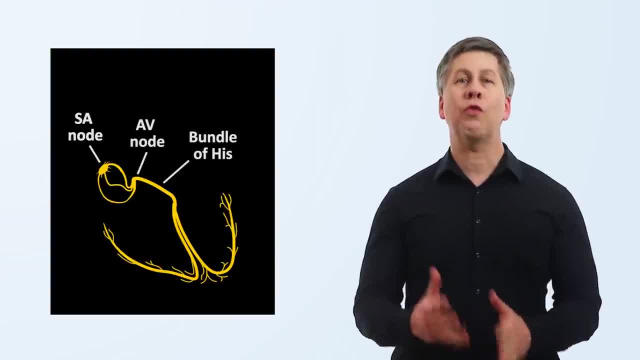 called the His bundle that divides into right and left bundle branches which travel to the right and left ventricles respectively. The right and left bundles terminate in a network called the Purkinje fibers, which rapidly deliver the signal to the ventricles. 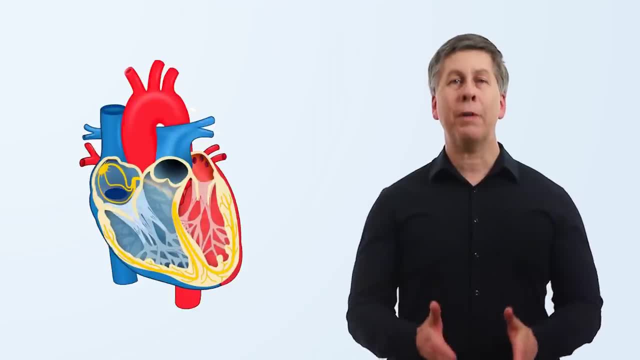 The overall consequence of this system is the rapid and nearly simultaneous contraction of the right and left ventricles in a wavefront that begins inferiorly at the cardiac apex and travels upwards towards the valves, which helps to increase the efficiency with which the heart ejects blood. 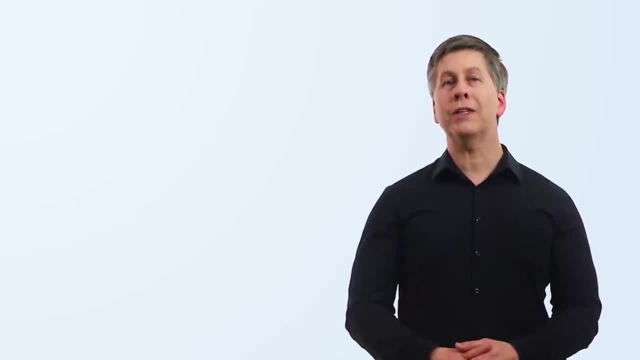 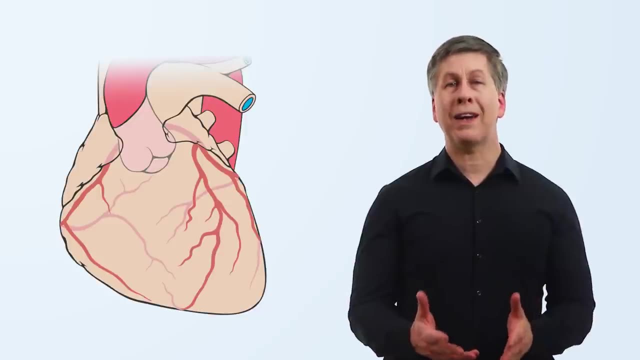 To see the coronary arteries, that is, the arteries that supply the heart muscle itself, we need an exterior view And again, the limitations of two dimensions make it impossible to see all of them at once- Coming off the aorta immediately above the aortic valve. 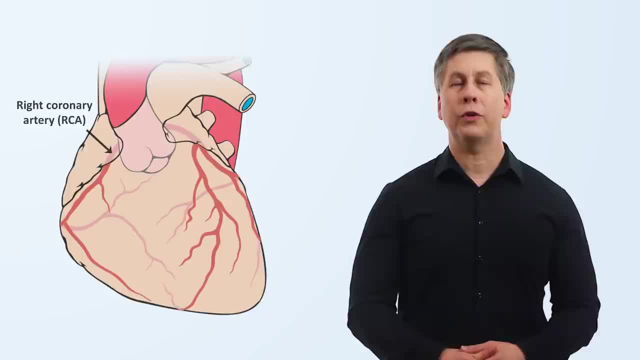 are two coronary arteries. One is the right coronary artery, or RCA, which predominantly supplies blood to the right ventricle and usually to the SA and AV nodes of the conduction system. The other is the left coronary artery, more commonly known as the left main coronary artery. 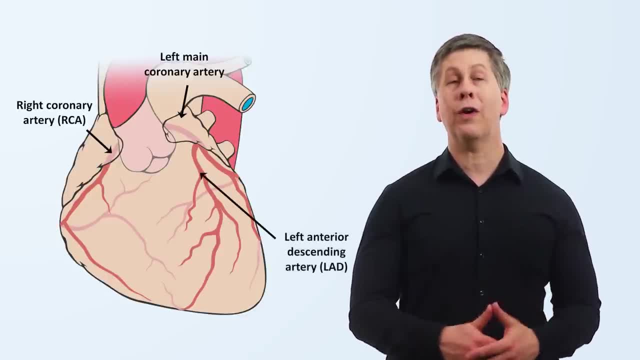 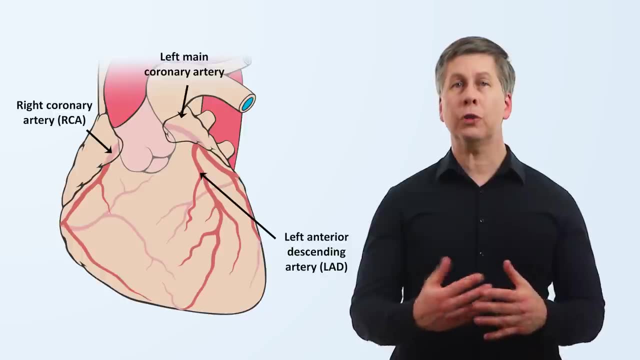 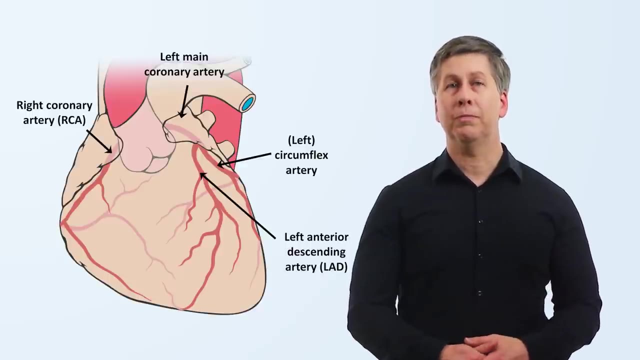 which quickly bifurcates into the left anterior descending artery, or LAD, which supplies the anterior interventricular septum and anterior wall of the left ventricle, and the left circumflex artery, which wraps around the hind, to supply the lateral wall of the left ventricle. 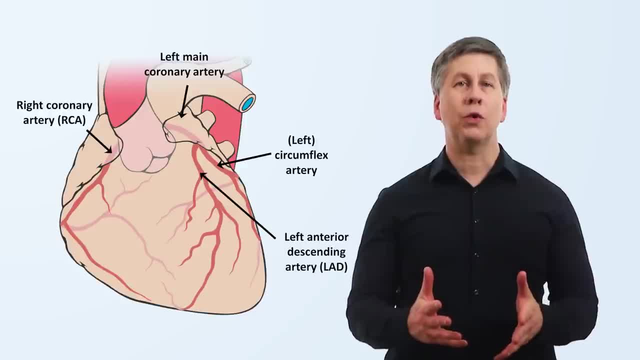 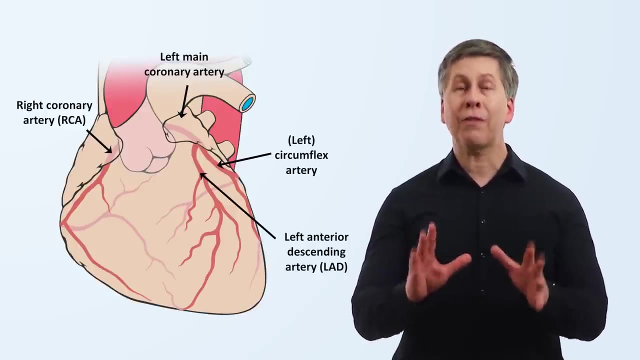 The coronary circulation contains a number of anastomoses or distal connections between these three arterial territories that allow for some redundancy of blood supply in the event that one artery becomes obstructed. Also, there are many normal and pathologic anatomic variations. 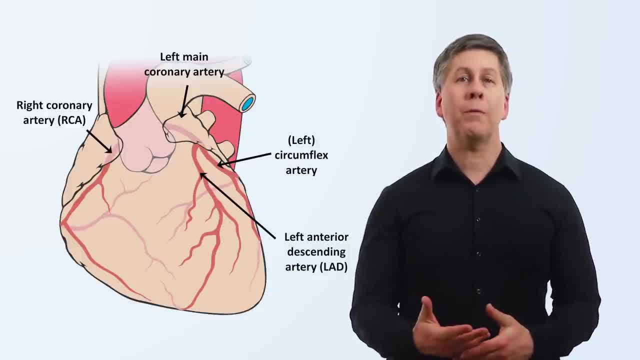 to the coronary circulation, most notably the normal variations in how blood is supplied. For example, the coronary circulation of the left ventricle is supplied to the posterior interventricular septum and the inferior wall of the left ventricle, As I mentioned. 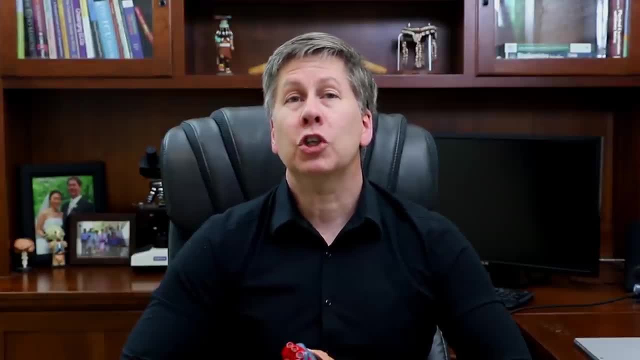 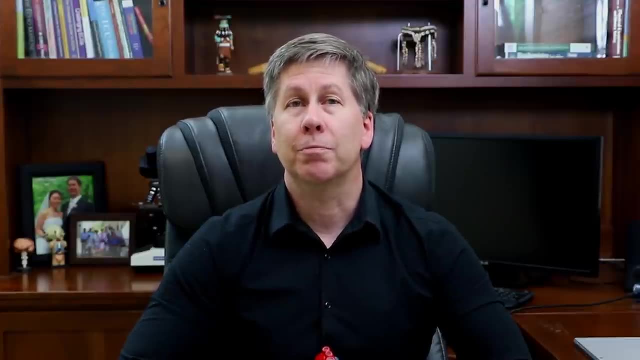 the heart is a difficult organ to accurately represent anatomically in two dimensions, So therefore I'm going to show you what it looks like in three dimensions, so you can get a better idea of how different cardiac structures relate to one another. Here is the exterior of the heart. 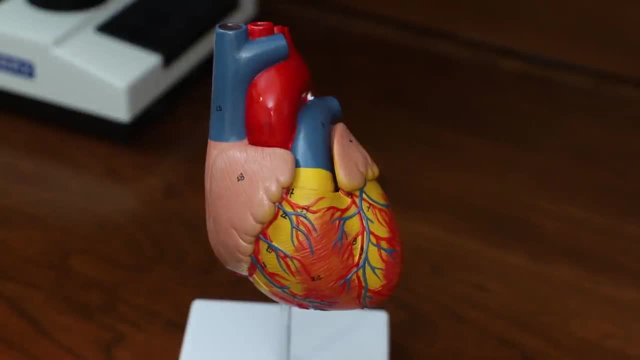 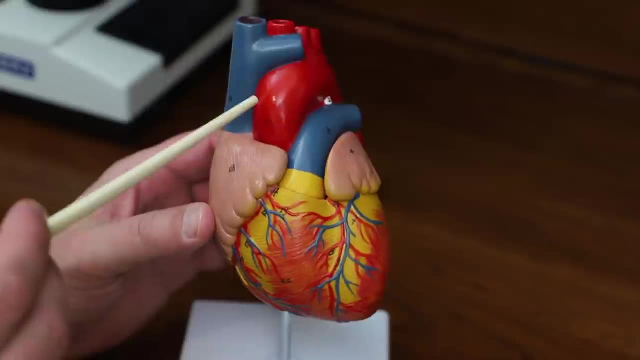 We can start with the great vessels and we can immediately see the very close proximity to one another. Here is the SVC or superior vena cava, Here is the aorta which loops upwards and posterior into the aortic arch And here is the main pulmonary artery. 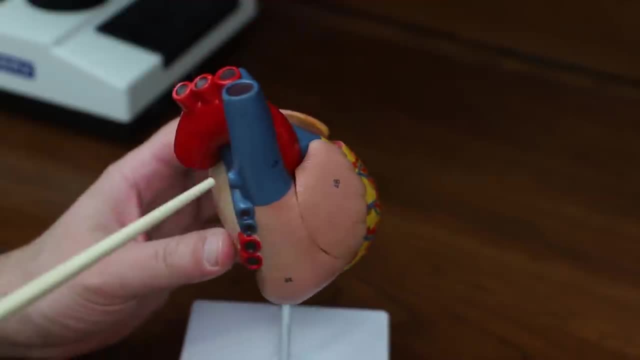 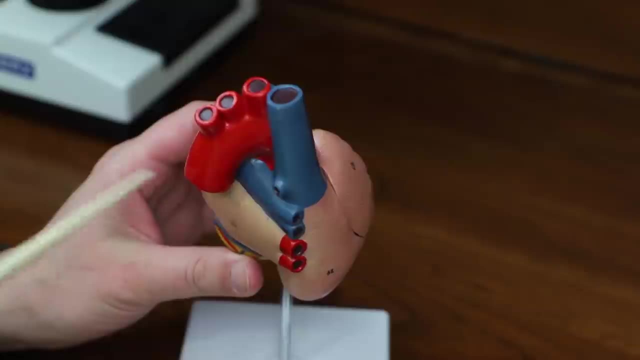 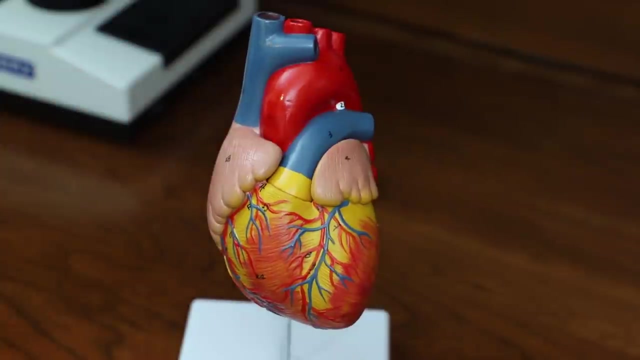 which bifurcates into the left and right pulmonary arteries. We can also see the four pulmonary veins as they enter the left atrium on the posterior side. Another structure apparent from the outside, one which I have not discussed yet, are funny-shaped things. 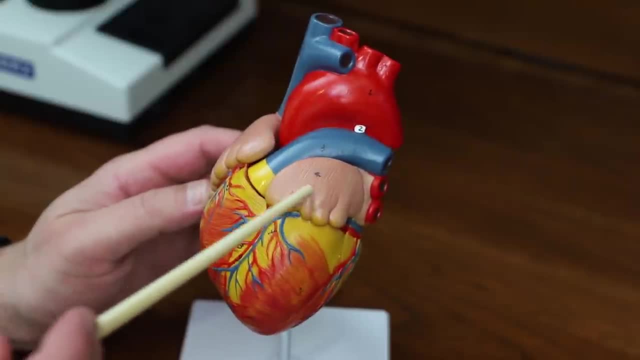 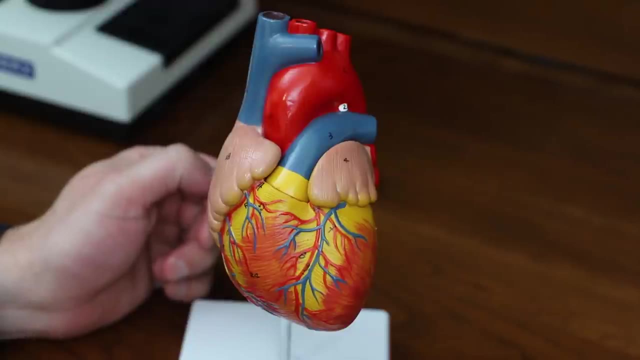 which extend a little over the surface. Anatomists call these the auricles of the right and left atrium, but most clinicians refer to these as the right and left atrial appendages. These are important, particularly the left atrial appendage. 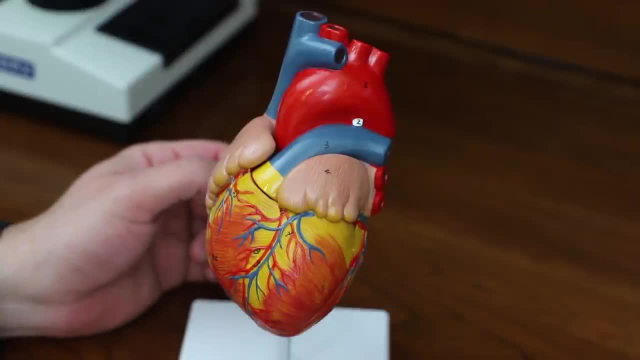 because these outpouchings are a region of relative stasis for blood and therefore they can be the site of blood clot formation, particularly during abnormal heart rhythms in which the atria do not contract, such as one called atrial fibrillation. 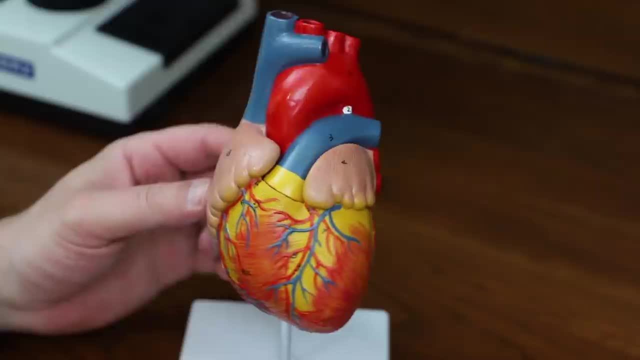 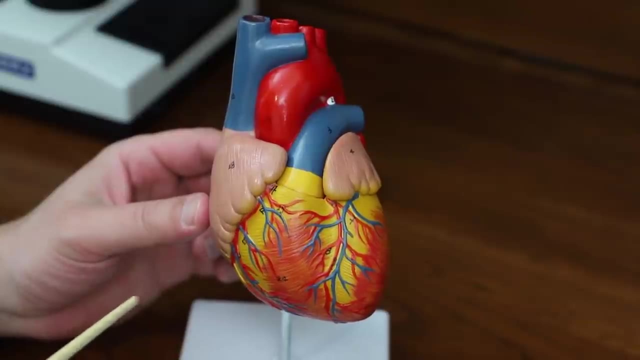 On the outside we also see the coronary vessels. This one here is the right coronary artery which supplies the right ventricle. The left main coronary artery is hidden behind the pulmonary artery, as is its bifurcation, but here is the left anterior descending artery. 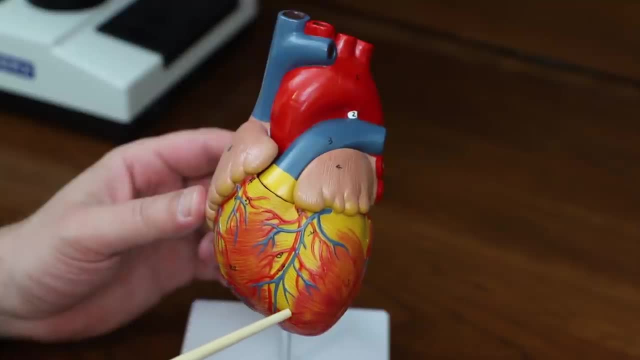 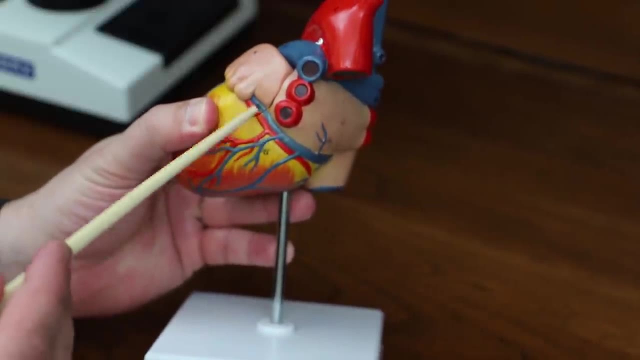 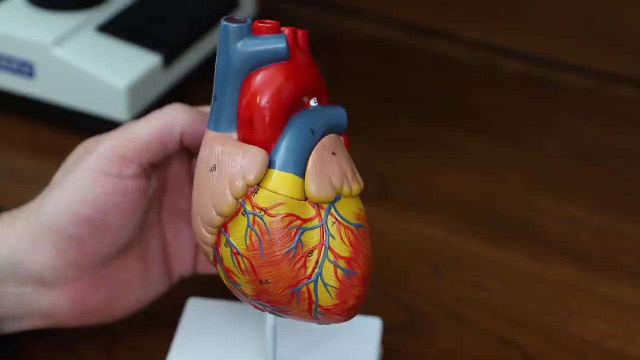 supplying the anterior wall of the left ventricle and around the back is the left circumflex artery supplying its lateral wall? I had mentioned that there were a large number of variations to coronary anatomy, including which artery supplies blood to the inferior wall of the left ventricle. 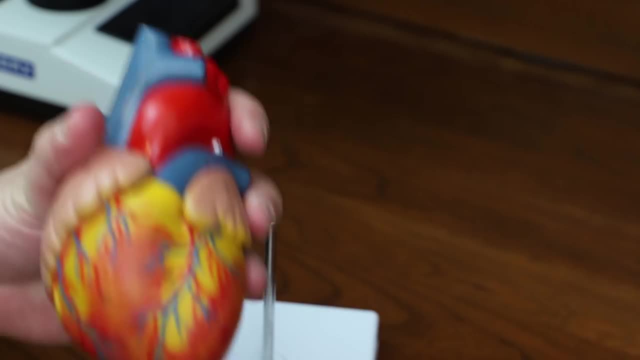 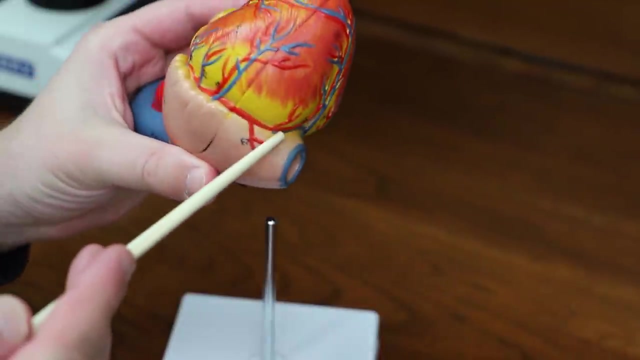 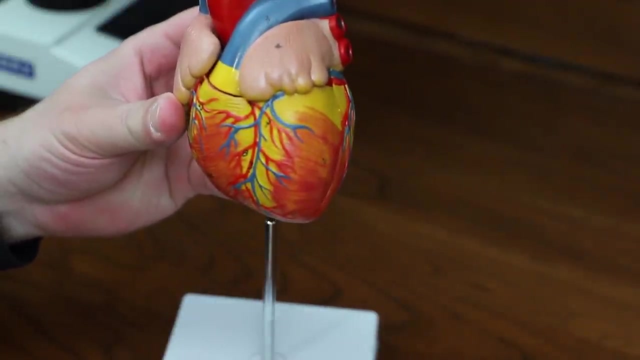 In this case, if we follow this vessel right here backwards, we'll see that it originates from the right coronary artery. so therefore this is called right dominant circulation. The last thing to note on the outside is this blue vessel right here. 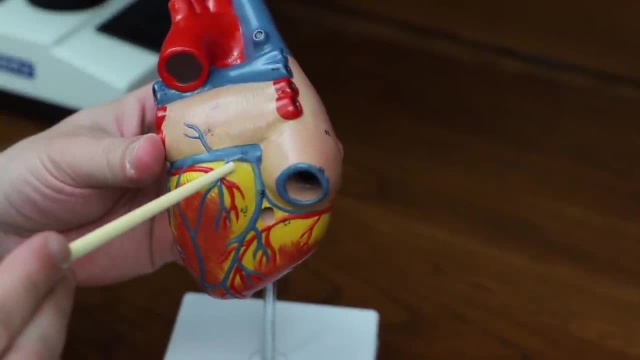 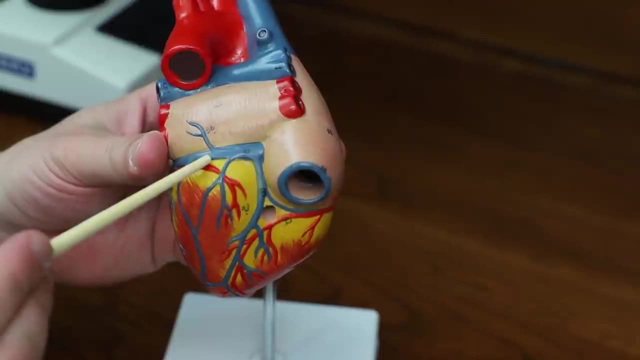 which, at its most distal end, is known as the coronary sinus, which drains blood from the heart itself into the right atrium. Now let's take a look inside. A few things to note here. First are the valves, specifically how close together they are. 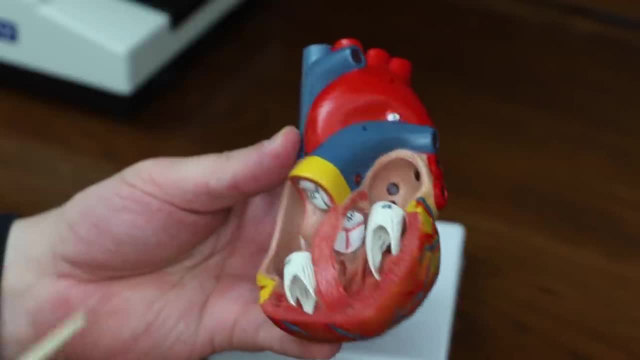 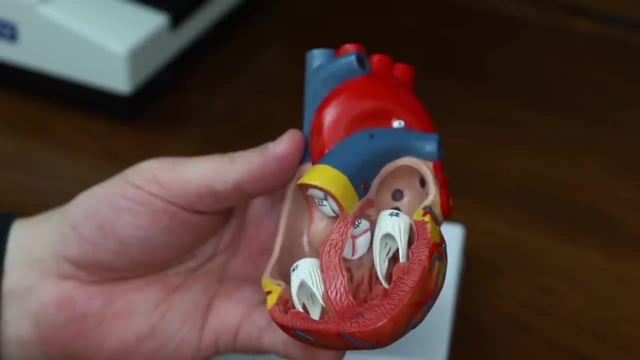 particularly the aortic and the mitral valves. These white extensions are the chordae tendineae. We can also better appreciate the difference in size and shape between the two ventricles, The right ventricle, which is down here, inferior to the tricuspid valve. 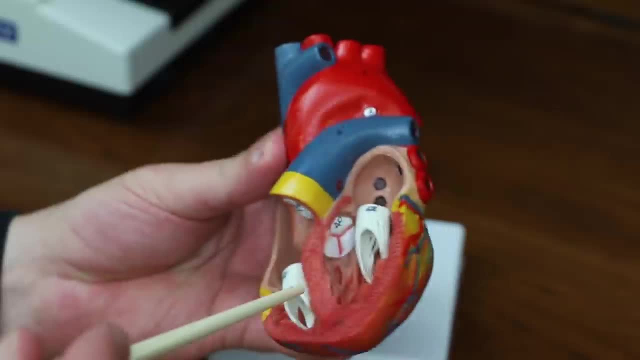 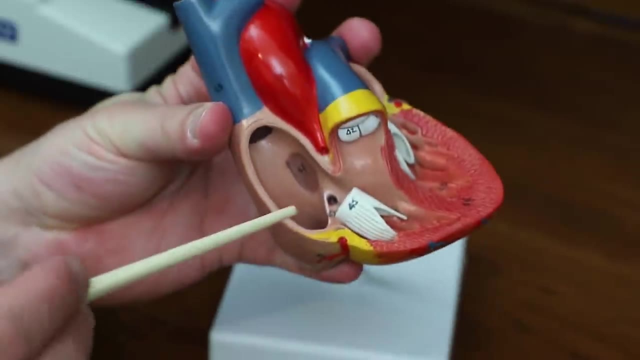 is relatively small and moon-shaped, while the left ventricle is slightly larger and a little bit more round. We also can see here: just superior to the tricuspid valve is the entrance of the coronary sinus. where the coronary sinus drains. 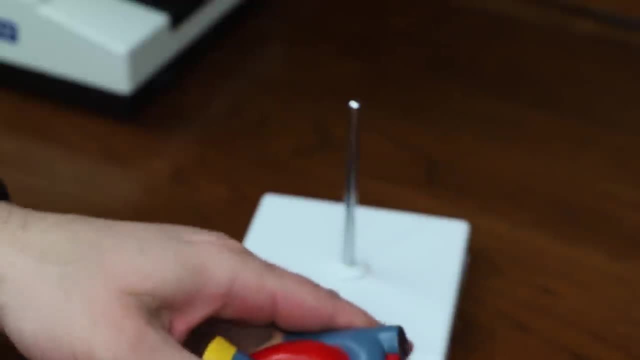 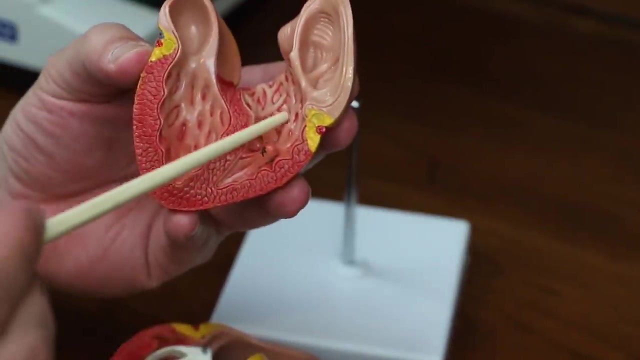 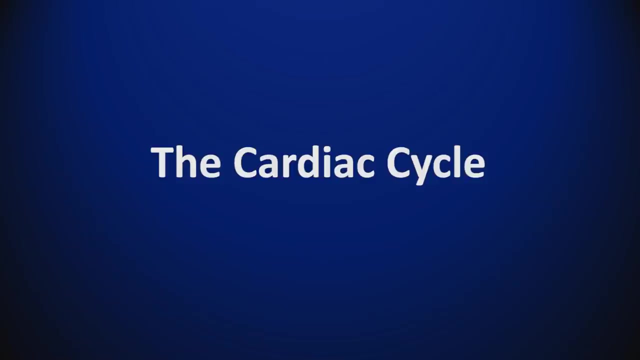 into the right atrium. On the inside surface of the ventricles we can note this mesh of muscular bundles. here These are known as trabeculations, and it's actually not known what function they serve. The cardiac cycle is the sequence. 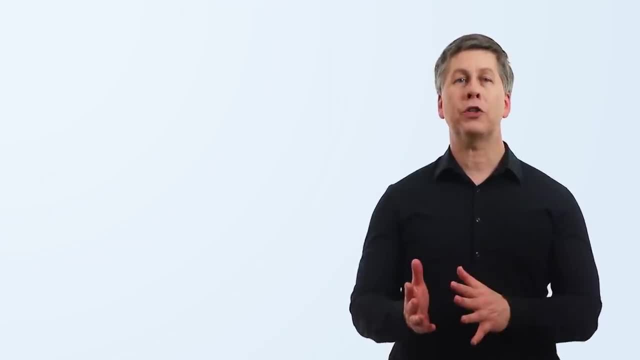 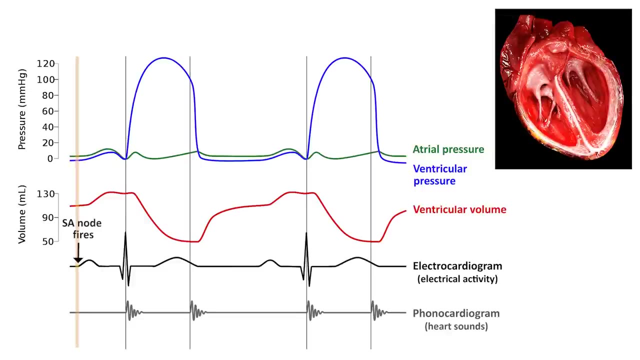 of all events within the heart that occur from one heartbeat to the next. Each cycle is triggered by the SA node firing an electrical signal. This signal triggers the right and left atria to contract, squeezing blood through the already open tricuspid and mitral valves. 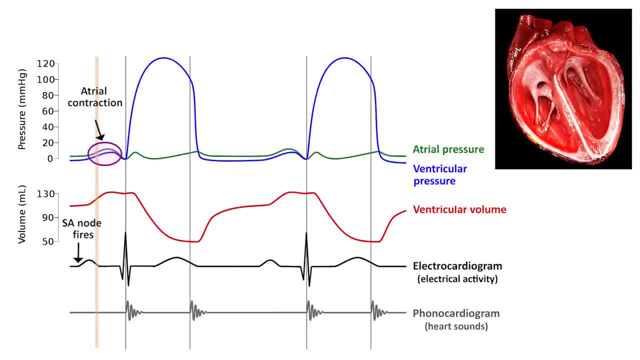 into the right and left ventricles. This period of atrial contraction is formally referred to as atrial systole, but is more commonly referred to as the atrial kick, After the electrical signal reaches the AV node and undergoes the brief AV delay. 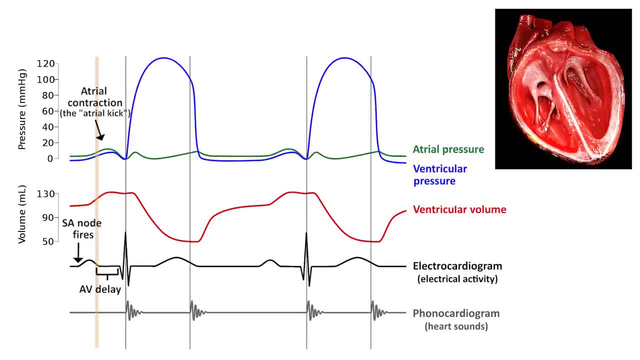 allowing time for filling of the ventricles during the atrial kick. the signal propagates through the hispochondriac system and triggers ventricular contraction. as we've already discussed, The rapid increase in pressure within the ventricles causes the AV valves to quickly snap shut. 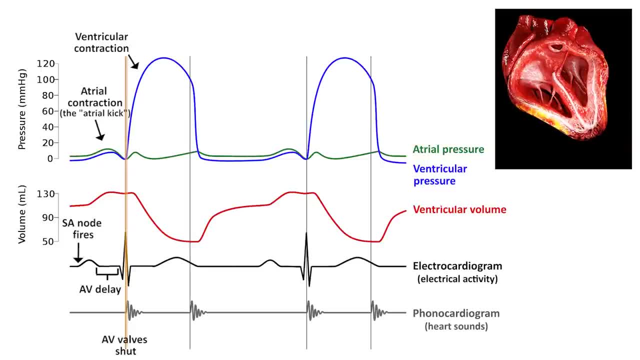 triggering the first heart sound in the classic lub-dub of the heartbeat. This first heart sound is known as S1, and the intraventricular blood is ejected through the now open semilunar valves. After a brief period of time, the ventricles relax again. 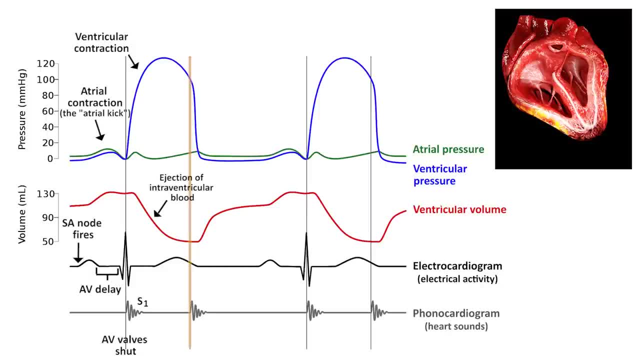 At this point, there is higher pressure in the pulmonary artery and aorta than in the right and left ventricles respectively, so the semilunar valves snap shut, resulting in the second heart sound, known predictably as S2.. At this point, 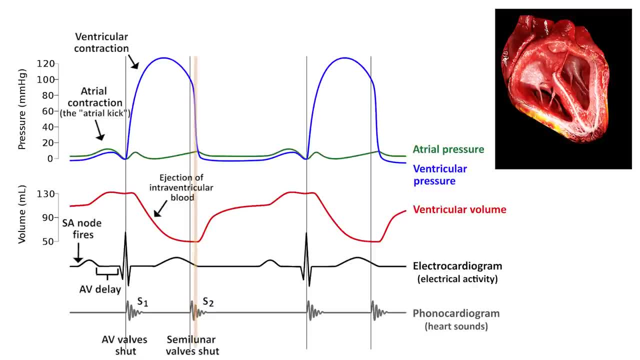 the ventricles have emptied much of their blood and relaxed to the point that the pressure in the atria are now higher than in the ventricles, and so the AV valves open once again, and this pressure gradient drives the passive filling of blood. into the ventricles even before the next SA node. impulse triggers atrial contraction. This is a very common case, where the ventricles contract during the cycle of the cycle, and the period of the cycle during which the ventricles are contracting is called ventricular systole. 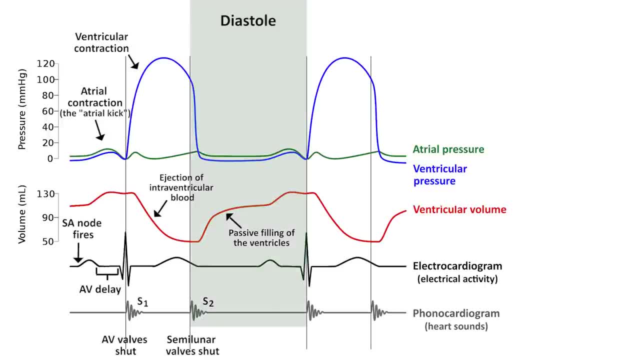 or usually just systole, and the period of the cycle during which the ventricles are relaxing is called ventricular diastole or just diastole. Confusingly, the timing of ventricular diastole includes atrial systole. 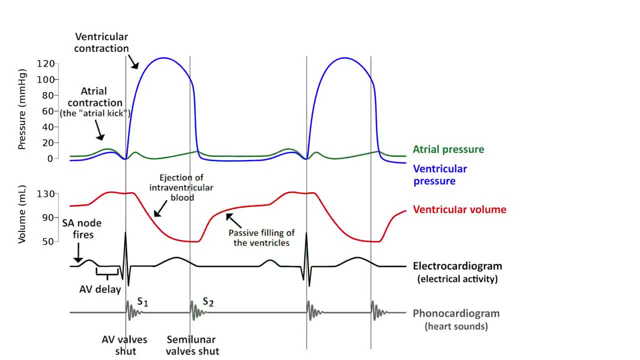 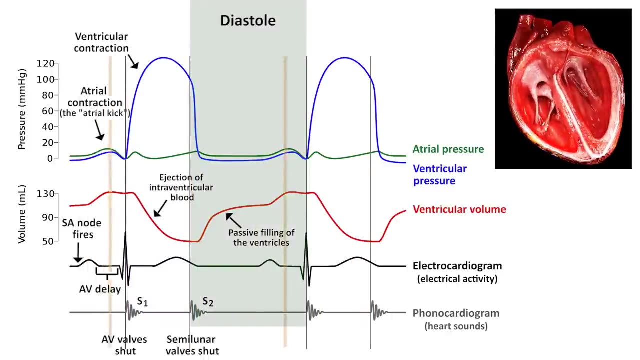 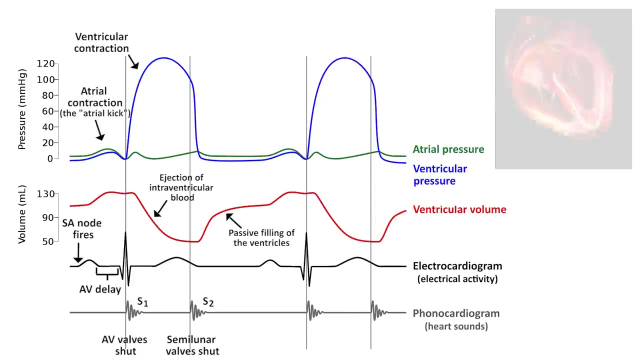 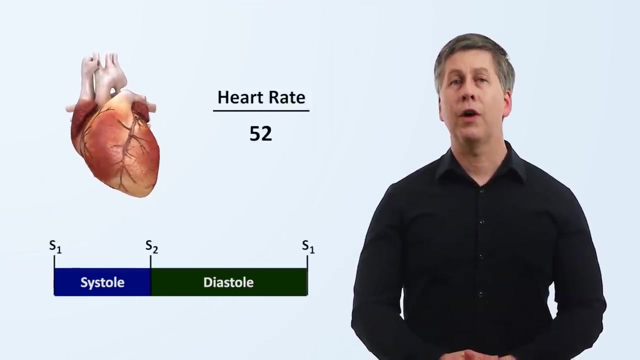 or sometimes just atrial contraction And blood. blood is moving from the atria to the ventricles throughout all diastole, so both before and during atrial contraction. The final point about the cardiac cycle: systole is always shorter than diastole. 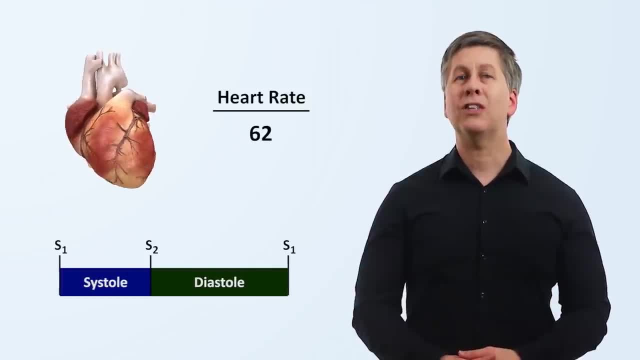 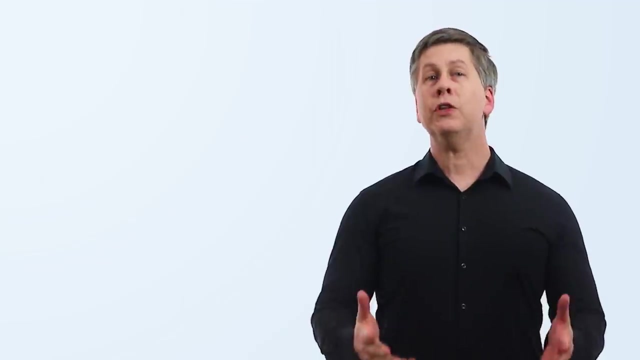 although the relative fraction of the cardiac cycle each takes up is dependent on the heart rate, As the heart rate increases, diastole shortens, much more so than systole, such that at extremely fast rates, they can be almost equal in duration. Up until now. 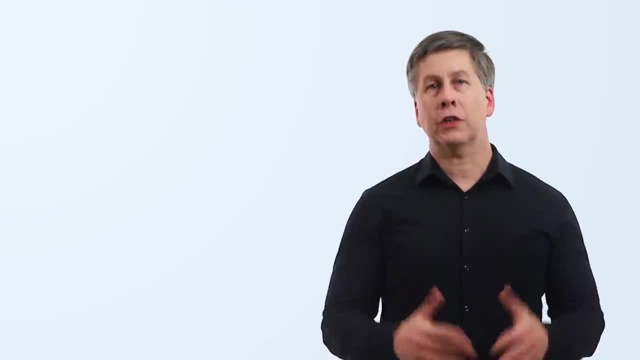 we were discussing the heart, but the heart is only one half of the cardiovascular system. The other half is the blood vessels, which are the conduits through which blood is pumped around the body, moving from the heart to the peripheral tissues and from the peripheral tissues. 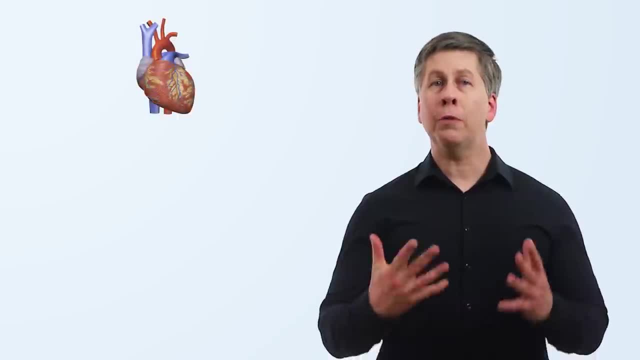 back to the heart. There are five basic types of vessels. Starting from the heart, all blood leaves the left ventricle via the aorta. From the aorta branch off large and medium sized arteries and smooth muscle, allowing them to handle high pressure. 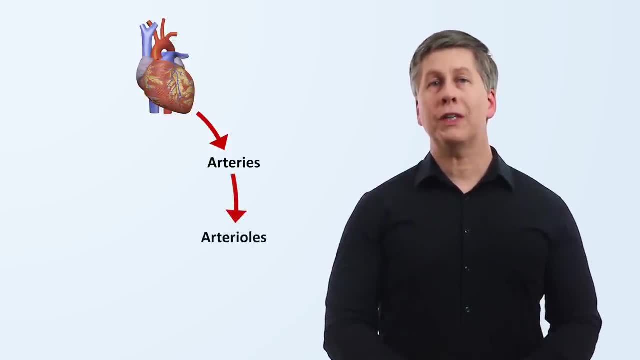 Arteries divide into smaller arterioles, which are the site of greatest resistance to blood flow through the circulation, And arterioles eventually divide and divide again into microscopic networks of extremely small vessels called capillaries, which are so small as to be lined. 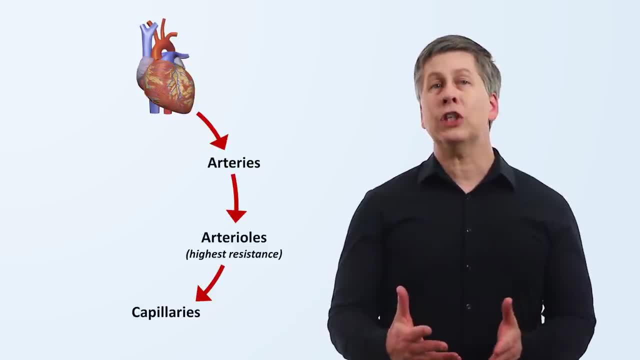 by a single layer of endothelial cells. sometimes The capillaries are where gas exchange between blood and peripheral tissues actually occurs. Although the capillaries are tiny, there are billions of them in the body, such that their net cross-sectional area is many times. 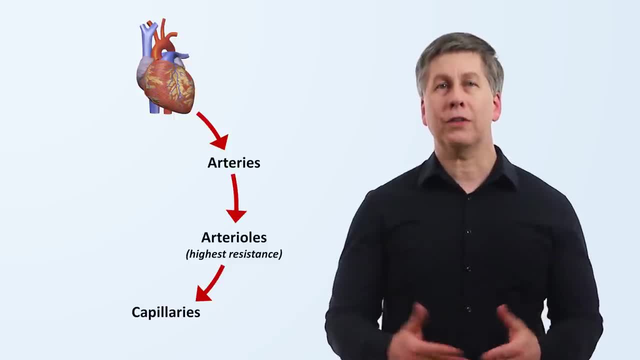 that of the aorta or of any other level of blood vessel. As a consequence, the capillaries are where blood travels the most slowly through the circulation, which is of course, helpful for the exchange of gas, nutrients and waste. After the capillaries: 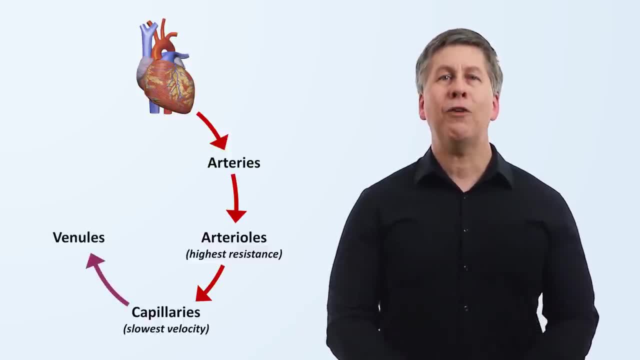 blood next moves to the venules, the arterioles and from there to the veins. In contrast to arteries, veins are relatively thin-walled and lack much elastic tissue, resulting in significant distensibility. This distensibility allows veins to act as a reservoir. 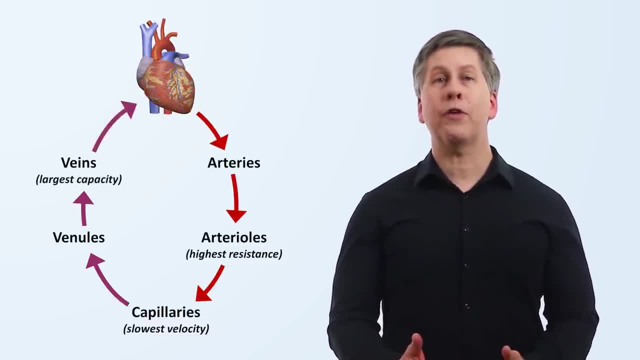 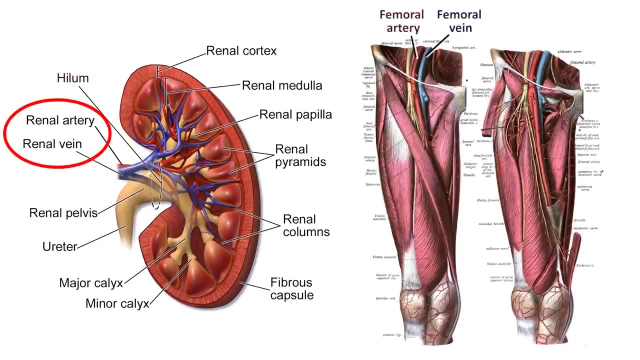 for blood volume. Arteries and veins are typically named for either the part of the body they travel through or which organ they bring blood to or away from, and they often exist as matching pairs. In addition to the blood vessels, there are also conduits. 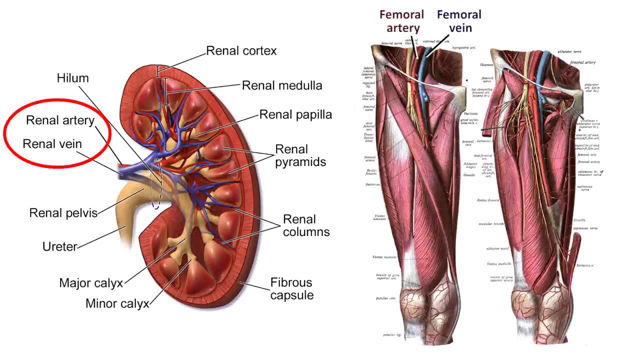 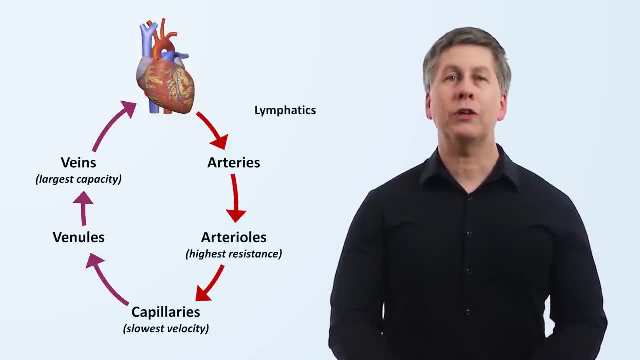 called lymphatics. Lymphatic vessels are responsible for returning interstitial fluid, that is, extravascular fluid that surrounds the cells and sits in the connective tissue- back to the bloodstream. Lymphatic capillaries merge into ever larger vessels until eventually. 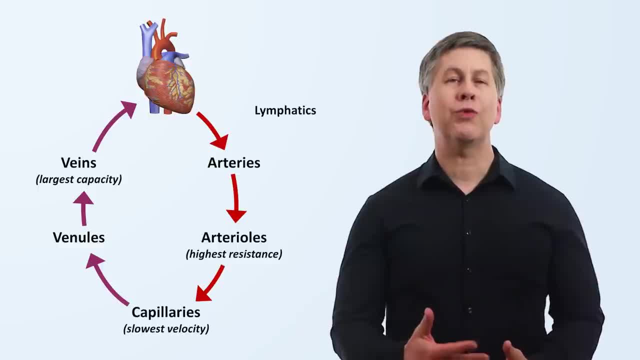 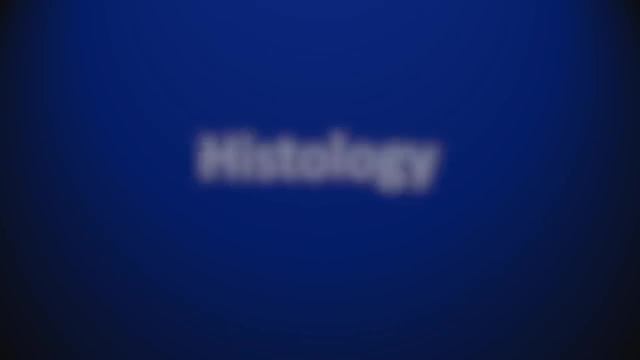 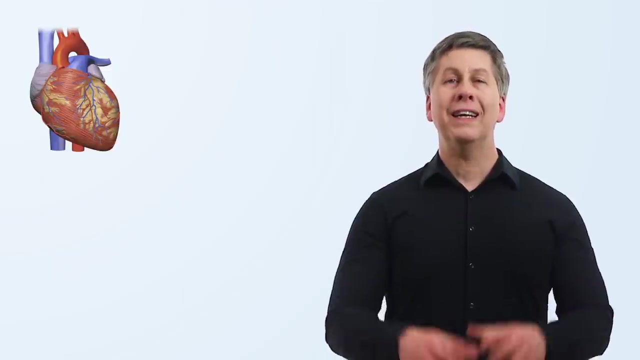 the blood vessels become interstitial. Lymphatic capillaries most feed into a conduit called the thoracic duct, which empties into large veins of the thorax. The last topic I'll discuss is histology and the microscopic structure of the heart. 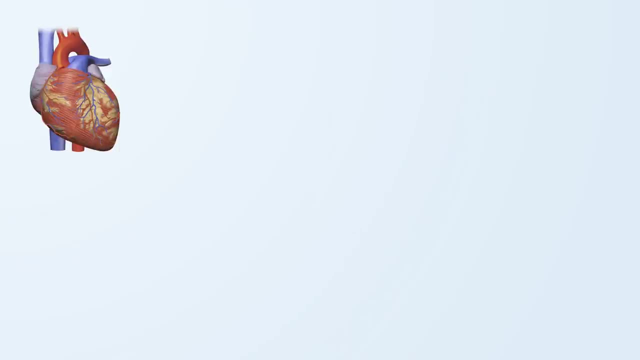 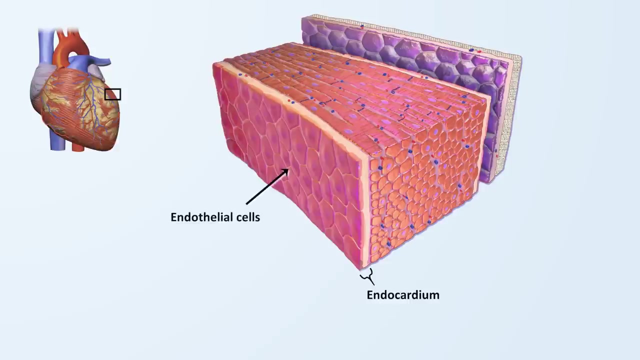 From a histological perspective, the heart is composed of three layers. First is the thin inner endocardium, partly composed of subendocardial cells similar to those that line the blood vessels. The endocardium also forms the lining of the heart valves. 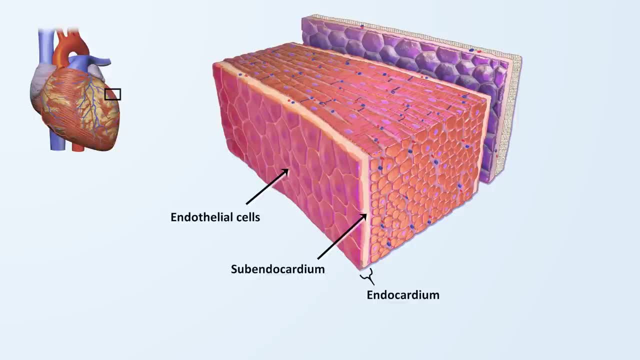 Immediately beneath the endothelium is the subendocardium, composed of loose connective tissue and is also the location of the Purkinje fibers. The next major layer is the thick myocardium, which is the heart muscle and which is composed predominantly. 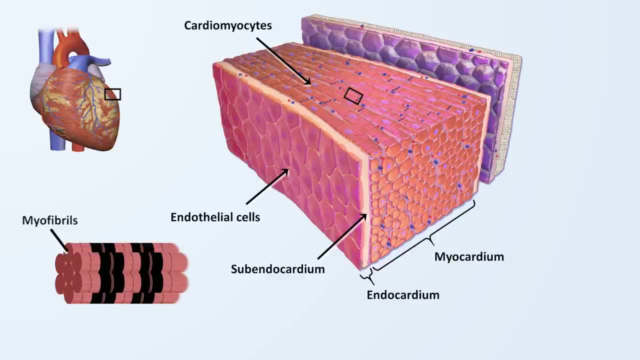 of long myofibrils that contain a repeating microstructure called sarcomeres, which are the fundamental contractile units of the cell. Within the sarcomeres are filaments of two proteins called actin and myosin, whose ATP and calcium-dependent 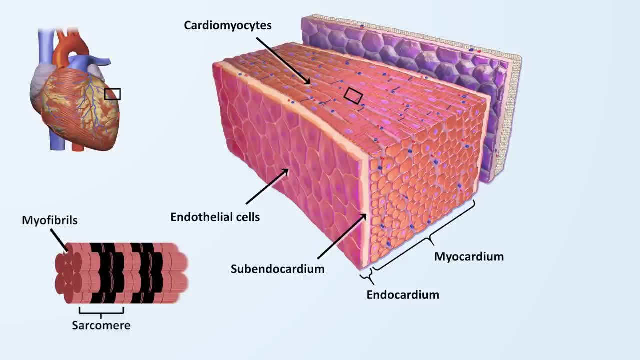 interaction is responsible for myocyte contraction. Cardiomyocytes contain a high density of mitochondria necessary for the continuous production of energy-containing ATP, Via porous bridges called intercalated discs, which allow for the free movement of electrolytes, which is necessary. 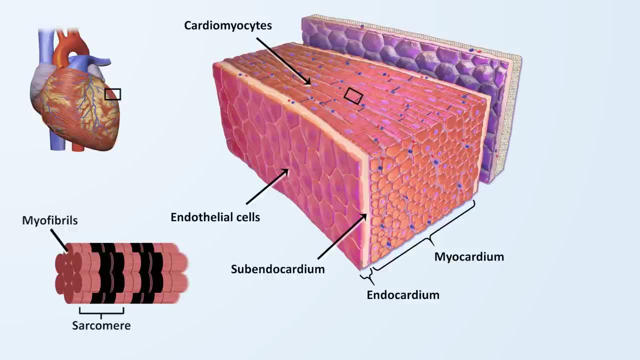 for rapid transmission of electrical signals from one cell to the next through the muscle tissue. This rapid transmission of signal is necessary for coordinated contraction. The overall process by which an electrical signal results in myocyte contraction is called excitation-contraction coupling External to the myocardium. 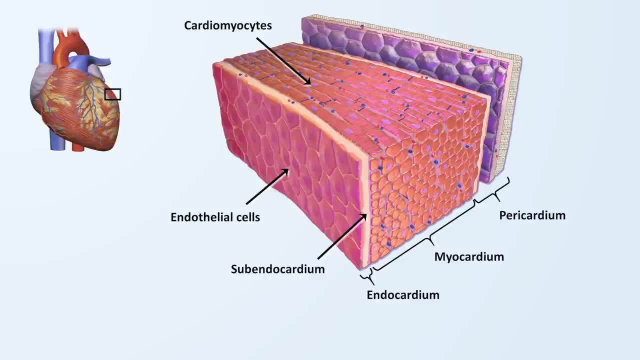 is the pericardium. The pericardium is a structure that encases the heart and the roots of the great vessels. It consists of a tough outer, fibrous pericardium which is tethered to the diaphragm in the sternum. 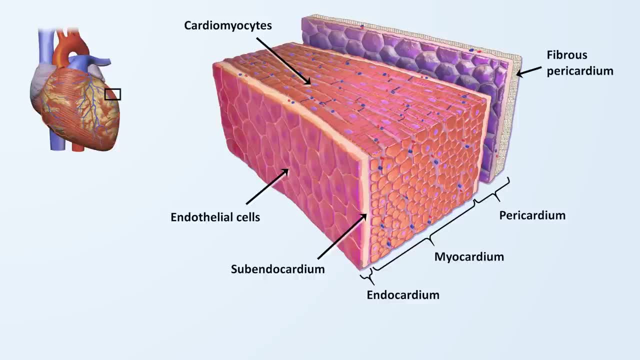 and which keeps the heart in place, And there is an inner, smooth, serous pericardium that's folded over on itself to make two separate layers containing a potential space between them. The outer of these serous layers is the parietal pericardium. 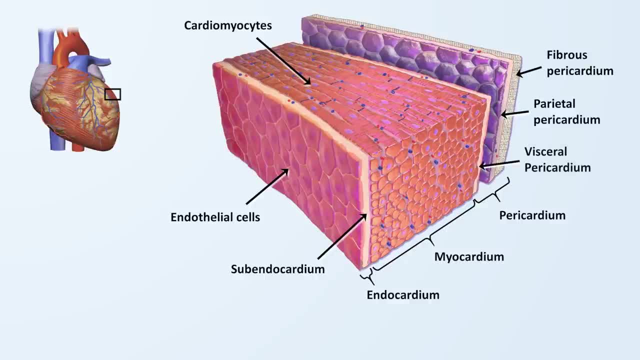 which is fused to the fibrous pericardium. It relies on the myocardium and is sometimes referred to as the epicardium. Yes, the terminology is frustrating. to keep straight, The potential space between the two serous layers is called the pericardial space. 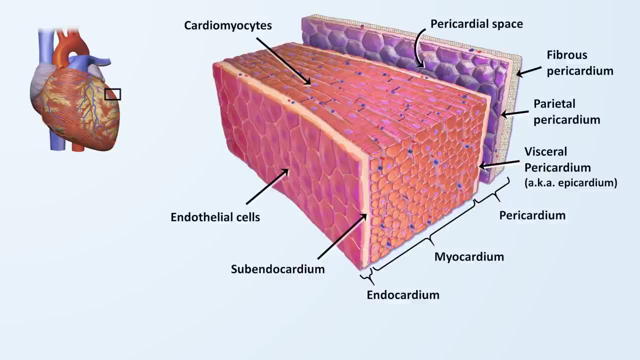 and is normally much thinner than it is in this image. It contains a thin film of fluid that allows the heart to beat in a near frictionless environment. However, in certain pathologic states, this space can significantly enlarge due to the pathologic excessive accumulation. 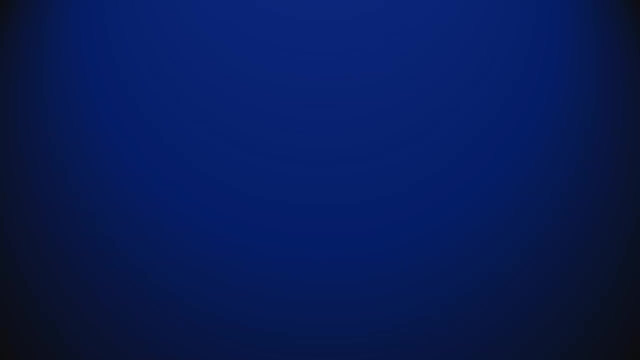 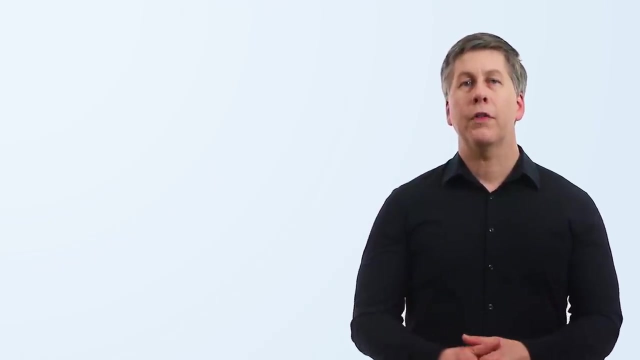 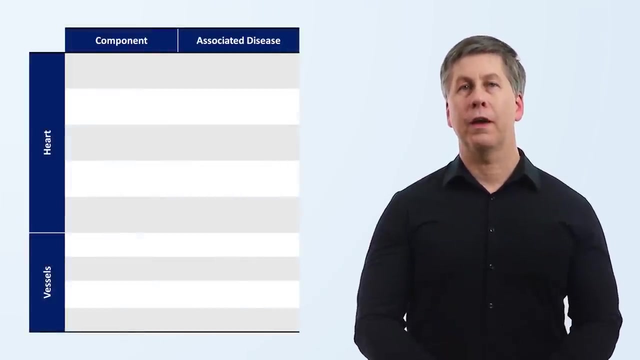 affecting cardiac function. To summarize what I've discussed so far, the cardiovascular system can be very broadly considered a collection of nine functional components, Five in the heart and four in the periphery, And pathologic conditions of the system can usually be mapped to just one of these components.